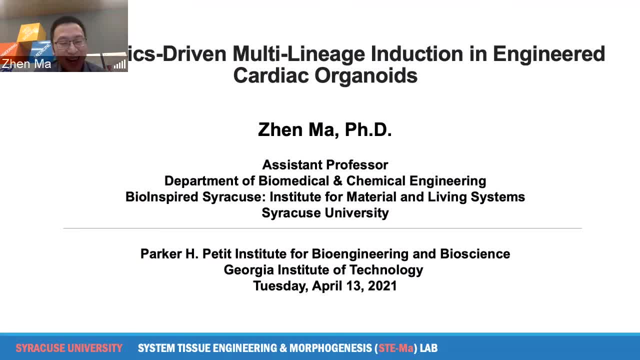 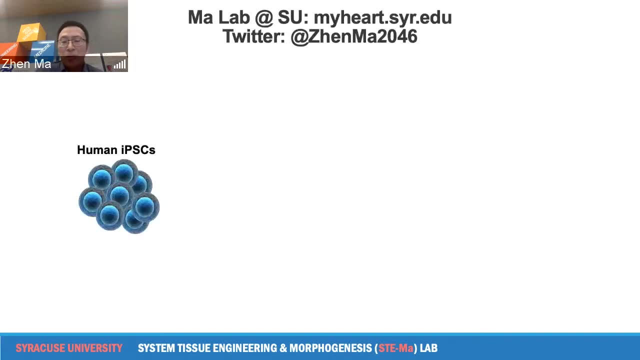 So in the next 45 minutes I'd like to share with some of our newest results on engineering stem cell organoids for specifically for drug screening purpose. So before we get into the real science, I'd like to take a moment to introduce my lab at Syracuse University. 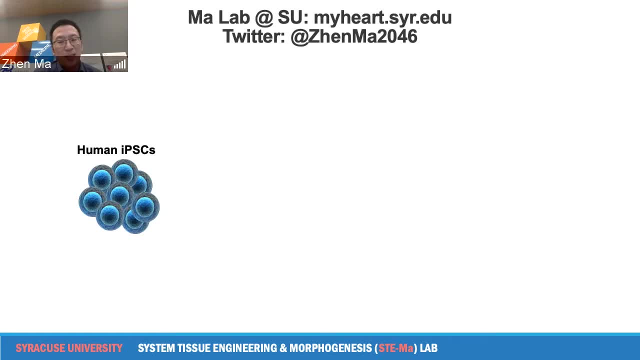 We take the advantage of human-induced pure component stem cell as a cell source to investigate different problems in biomedical science and engineering. We primarily generated three cell types: mesenchymal stromal cells, cardiomyelocytes and vascular endothelial cells from IPICs. 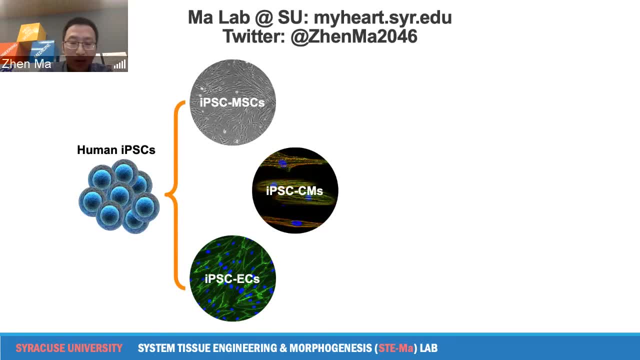 We're using all three of these cells. We're using all three of these cell types: mesenchymal stromal cells, cardiomyelocytes and vascular endothelial cells from IPICs. We're using our mesenchymal stem cells for bio manufacturing applications, from tissue fabrications to cell manufacture rings. 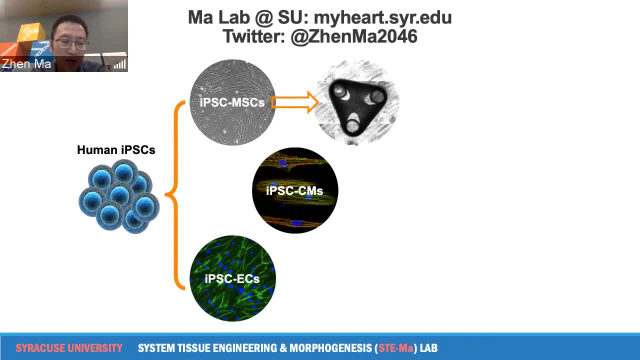 And now we are going to a little bit into act, without manufacturing rings, And we use our endothelial cells to study the formation of vascular structures in 3-D printed scaffolds, based on a collaboration with the Sab câmera Lab. latency And, of course, cardiac myocytes is our main focus of the lab. 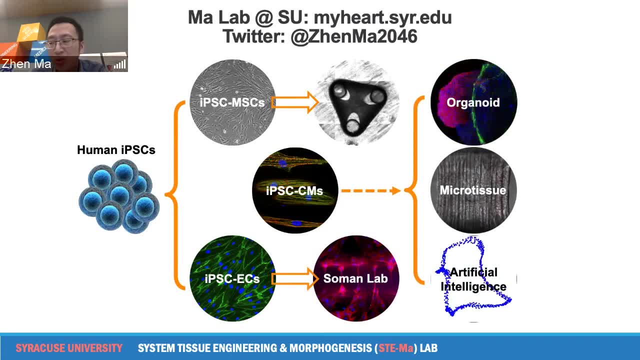 And with that we established two in vitro tissue models, including cardiac tissue models and cardiac microtissue models. We are also exploring some new directions to using advanced AI technology to better analyze the contractile functions of our organoids and microtissues as well. 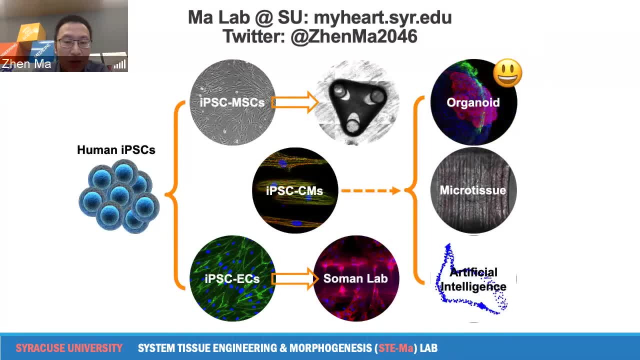 So in this talk I'm going to focus on our organoid model. I'd like to share some of our new results to see how these geometric confinements will affect organoid formation and the functions, And towards the talk. if I have time, I don't think I can touch a little bit on the new project on mesenchymal stem cell-stomach cell differentiations. 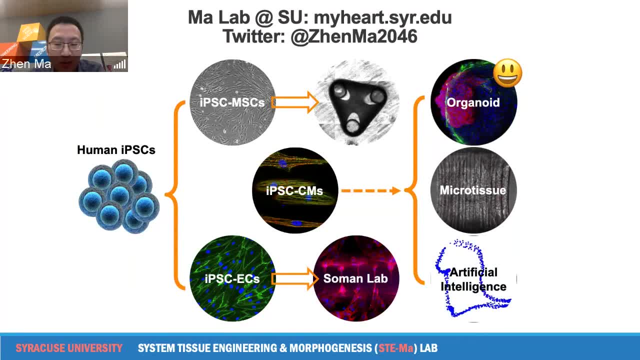 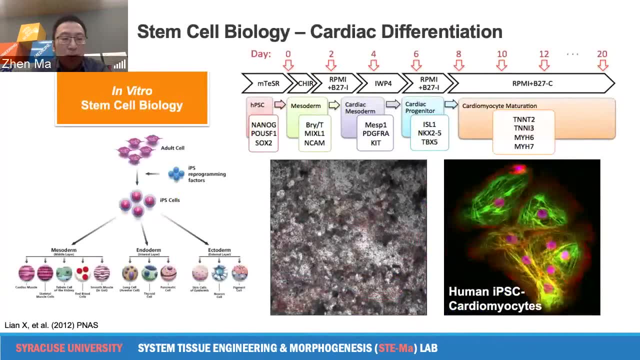 which we hope we can get into the field of cells. So, as I said, we're going to be focusing on the genomic cell and exosome manufacturing. So the advancement of human IPIC technology offers a really unique opportunities in regenerative medicine, Since we can differentiate many different cell types from IPICs for tissue repair and regenerations. 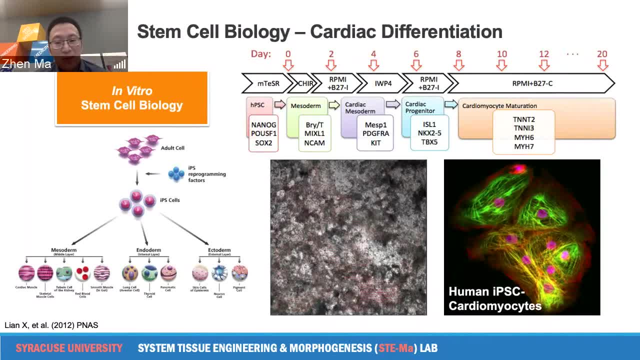 And specific for cardiac differentiations. we can derive cardiac myocytes with high efficiency. The different differentiation for particles is the different kind of cell types. follow this developmental cell biology with a cell-based transition from pyropotent stem cells to the mesodermal cells and then to the cardiac progenitor. 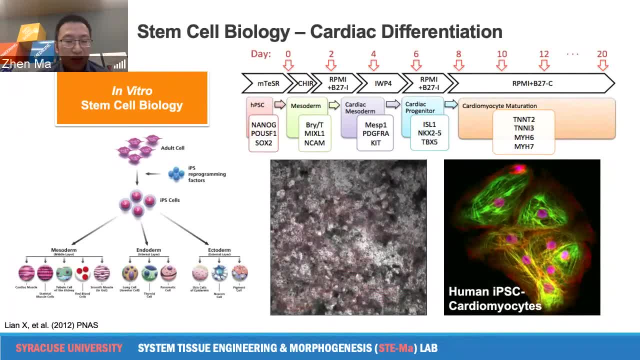 and finally become the working cardiac muscle cells. So, like you can see this, cardiac muscle cells can form a she-beating cell layer in the tissue culture plane and they also express key molecular feature signatures of cardiac mouse cells. Every time I show this beating video, I have to tell. 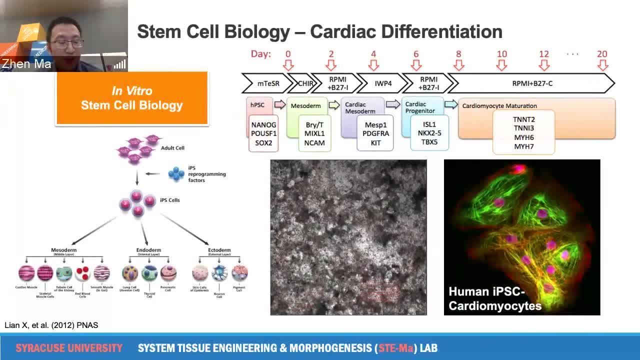 everybody that this is the best video we can get. if you see these such beatings from other presentations, This is probably the best reading they can get as well. So everybody claim they have really high efficiency. So on our hand- and I also talked about it before- the way that the neuroplasticity is achieved is by 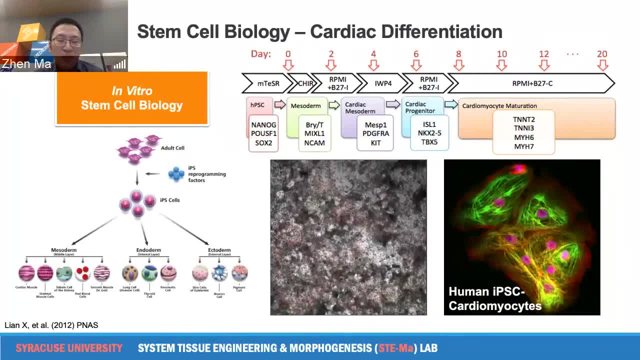 many people work on the cardiac differentiations. the efficiency is about like a 60 to 70 percent of cardiac male size productions. uh. so if you really want to get to uh like a high purity of the cardinal size, you have to using the pure purification particles. 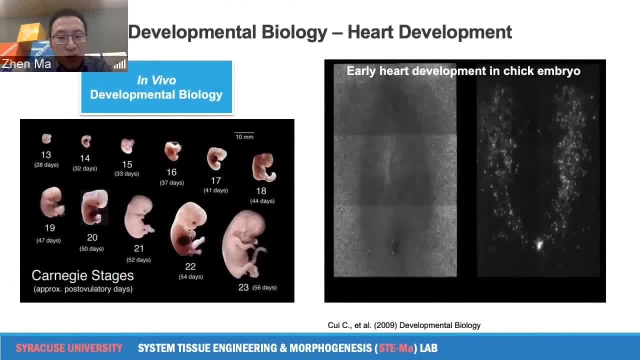 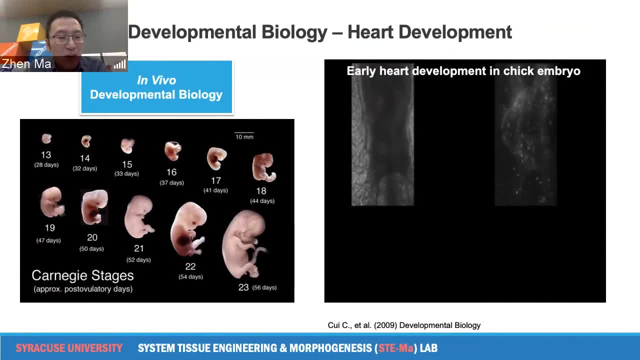 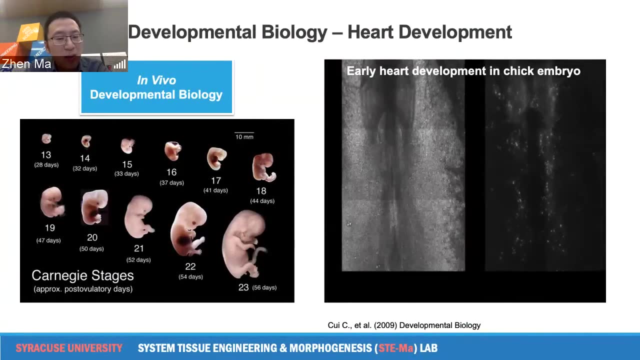 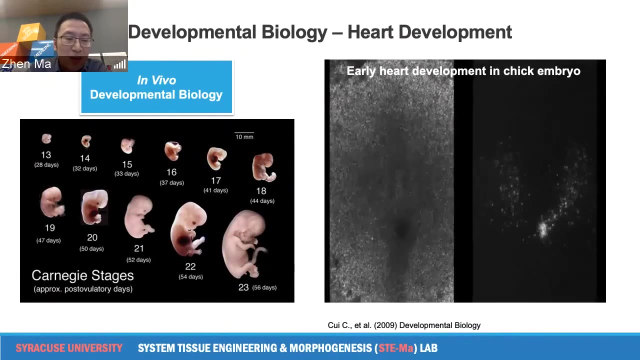 so, however, if we go back to the traditional developmental biology, which what is important here is not just a simple cell transition from one cell type to the others, but also the complex tissue growth and the tissue morphogenesis occurring throughout the impaired developmental process. again specifically to the heart development you can see in the video. 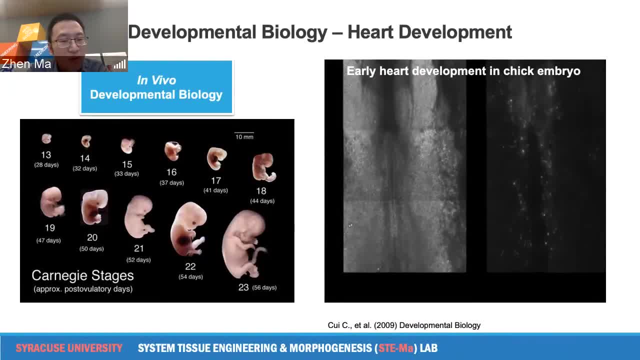 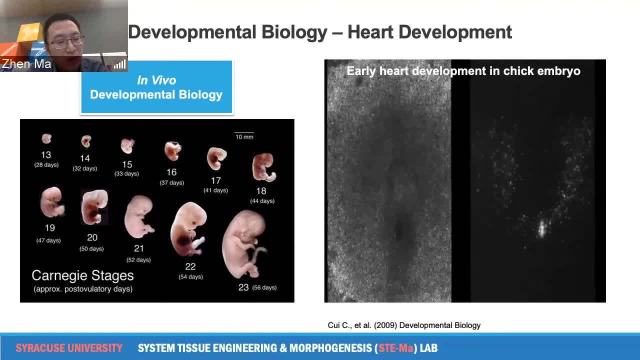 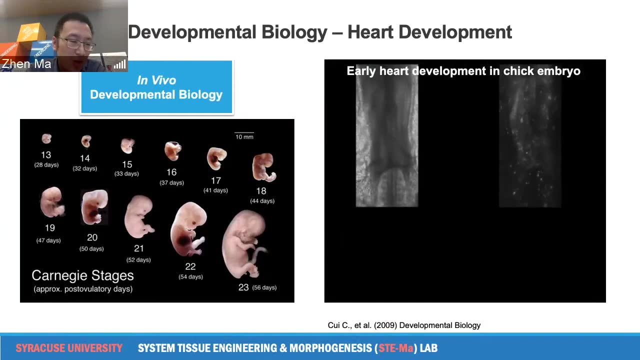 on the right is a cheek really around r formations isn't in that radius are the mesodermal cells migrate the long way to the center of the embryos and fills into the linear heart tube And this linear heart tube can loop and grow into the heart chambers. 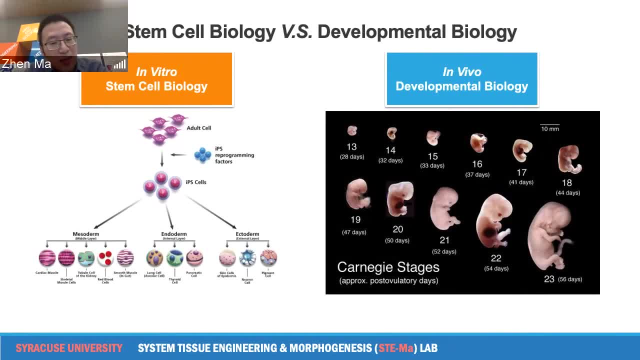 If we put this in vitro stem cell biology and the in vivo developmental biology together, there's many questions ahead of us And in my lab. particularly interesting two major questions: how the cell differentiate and the tissue morphogenesis coordinate to form complex tissue. 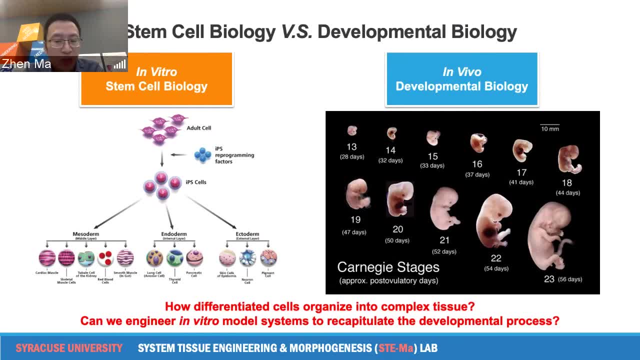 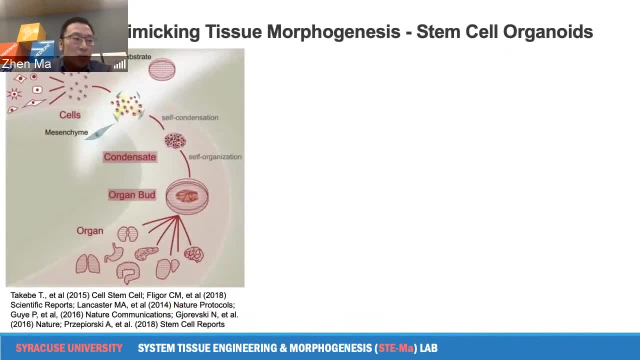 and how we can create an in vitro model system to recapitulate this developmental process. And these questions bring us to the stem cell organoid technology. So traditionally, people can grow the stem cell aggregates in sulfur hydrogels. in most cases it's matrigel. 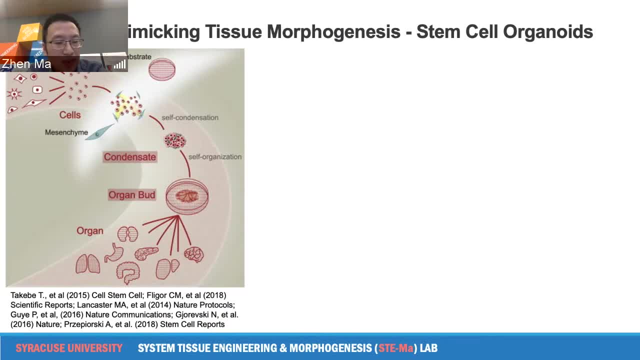 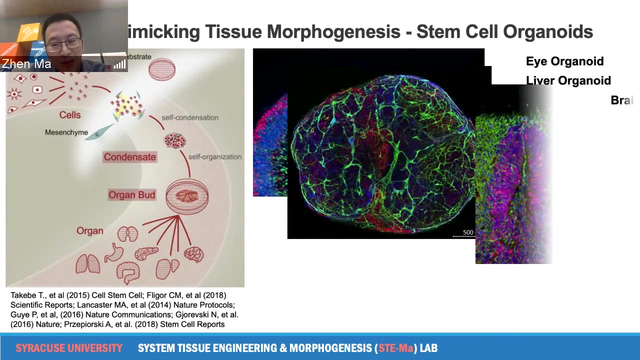 And induce the differentiation into a specific lineage And this is 3D aggregates can differentiate and develop into organoids that can mimic the early stage of a developing organ. There are many labs has been developing so many different tissue specific organoids And my lab is primarily work on the heart organoids. 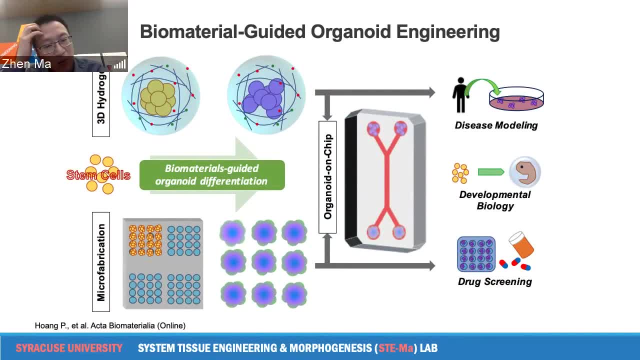 Meanwhile, as a bioengineer, we are seeking a better approach to control the stem cell differentiation and organoid production- This including growing organoids- within a synthetic hydrogel instead of a traditional matrigel, For example, PEG hydrogel has been used. 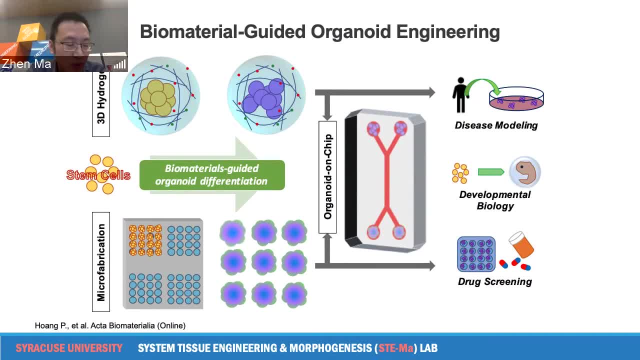 for organoid cultures. Dr Garcia has made a great contribution in this field. On the other side, micro-well and the surface, micro-patterning techniques has been also used to provide a controllable way to control the size, homogeneities and colony confinements. 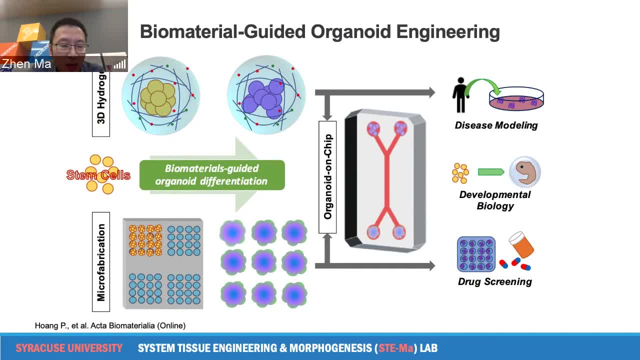 And these techniques can be also used for high throughput, scale-up productions of organoids for different applications And, more recently, integration of microfluidic systems and organoid cultures, where it is organoid, on chip platform for better control, The dynamic organoid. 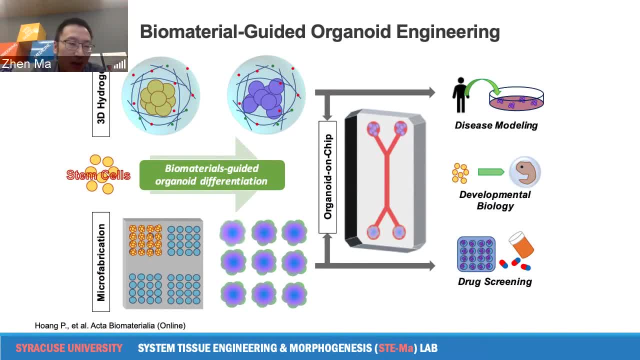 micro-environment and also give us a method or opportunities to study the multi-organoid interactions With all these technologies. the organoids has been used for different applications, For example disease modelings. people use it for fundamental development of biologies. 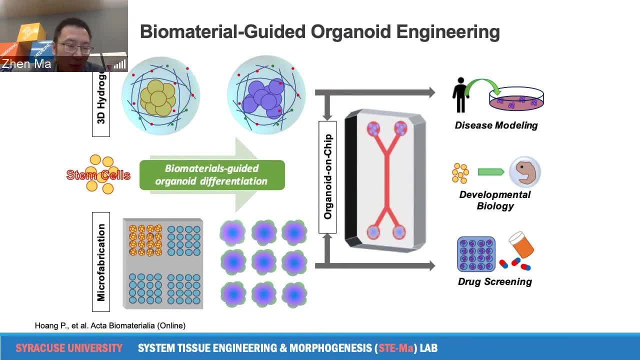 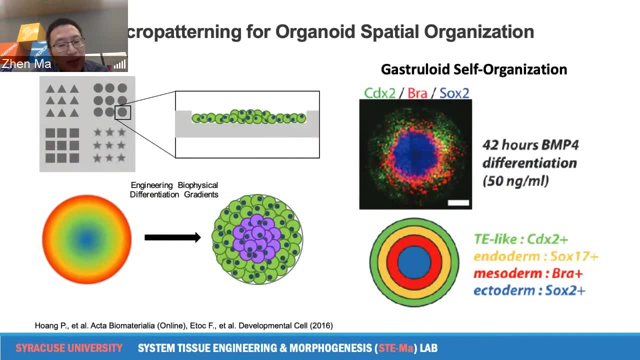 and also used for different drug screening applications. Specific to this micro-patterning technique for organoid productions, which we use for our hard organoids, we can create a different geometry of the path to pattern stem cell colony. The pattern surface will provide. 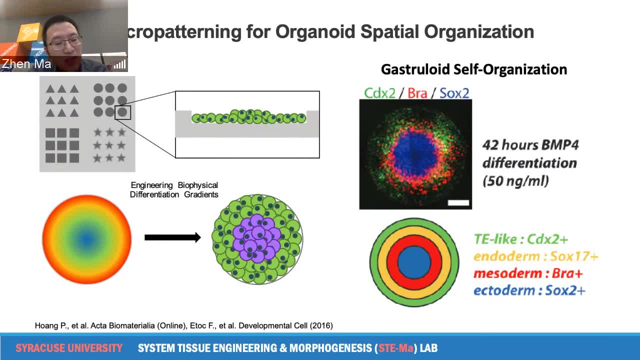 this, a geometric confinement to the cells, which can generate a gradient of a biophysical input from the edge of the patterns to the centers, And that gradient will drive the spatial differentiation of the stem cell. Showing you on the right is one- I think is the one of the best examples. 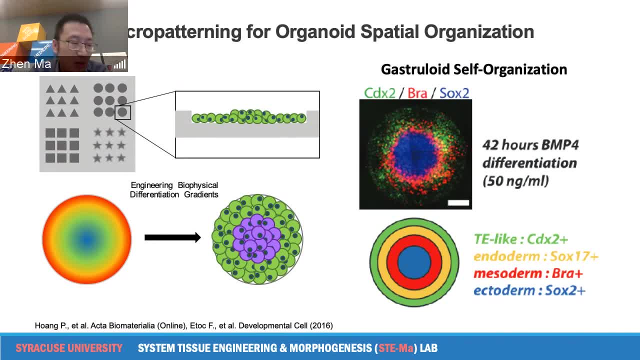 of micro-patterning techniques for spatial stem cell differentiation and organizations. So by micro-patterning the human embryonic stem cells into this circular shape and treating the cells with a P-morphogen BMP4. The EIC can differentiate on the cell of organization. 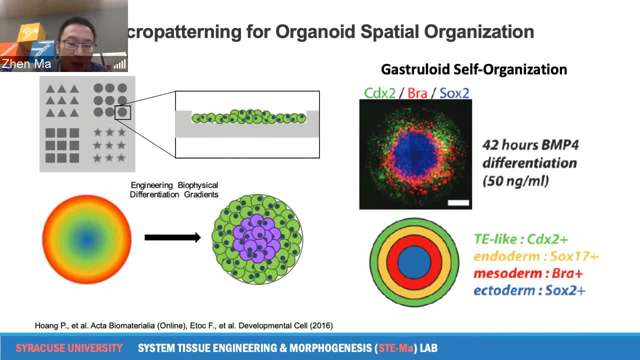 into this different layer of cells with trophoblast-like cells on the outside, and then next to it is endodermal layer, and then it's the mesodermal layers and then you have this echoderm layer in the center of the patterns. 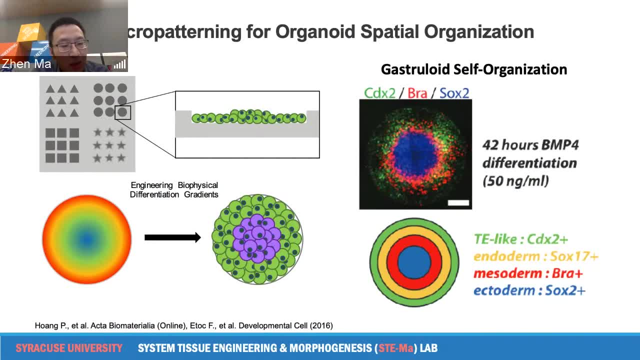 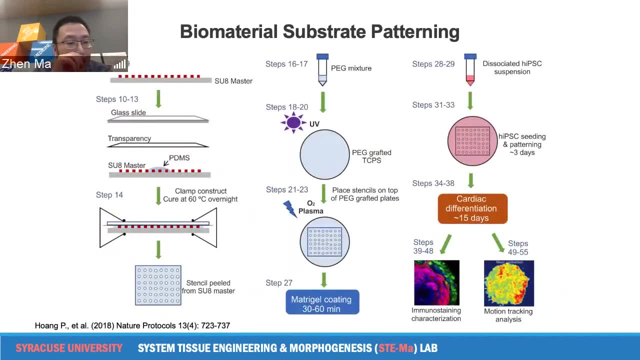 This spatial organization recapitulates this germ layer differentiation during the early embryogenesis. So in MATLAB we're using surface micropatterning method to grow alpha-cardio organoids. There's some more details in our published papers, but briefly, we grow a thin layer of a path. 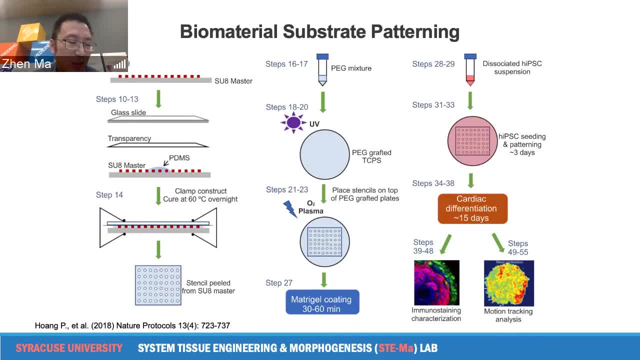 on the tissue culture- polystyrene in most cases, just like a 12-well plate or a six-well plate- and then we put a layer of a PDMX stencil on top of this PAG layer and the PDMX have a clear through hole. 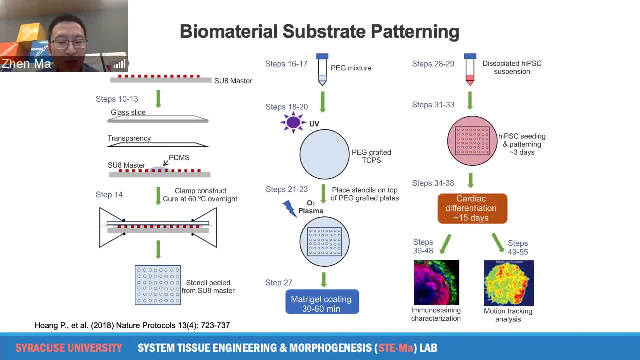 and where the hole is, we can use an oxygen plasma to selectively etch away the PAG layer underneath. So there's a region without a PAG layer and that region we can code in with matrigel and grow our IPICs. 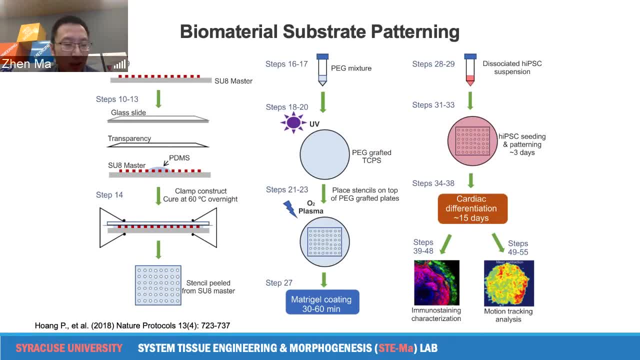 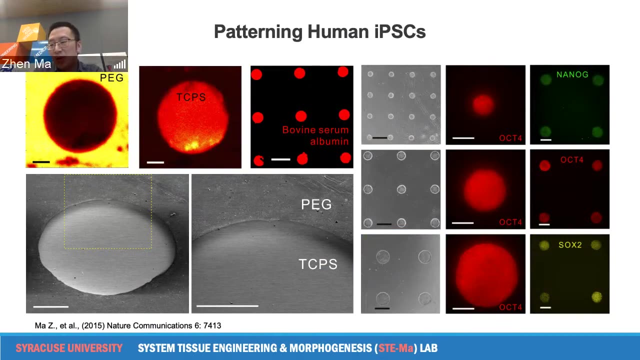 After we grow our IPICs, we just follow that traditional cardiac differentiation protocol to generate our cardiac organoids. So this is like surface chemistry we did. I did when I was in Kevin Feely's lab. So basically we can show where the PAG layer is. 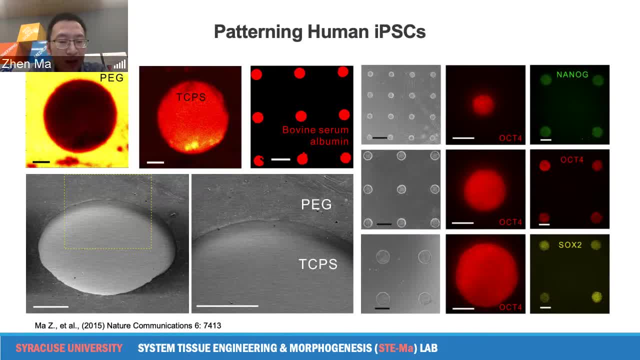 and where it's not, and we coded the pattern surface with matrigel And the matrigel can only deposit onto the region without pack, so we can grow our human iPSCs into these specific patterns with different size and shapes. We also show that iPSCs can maintain their pure potency after micropythening procedures. 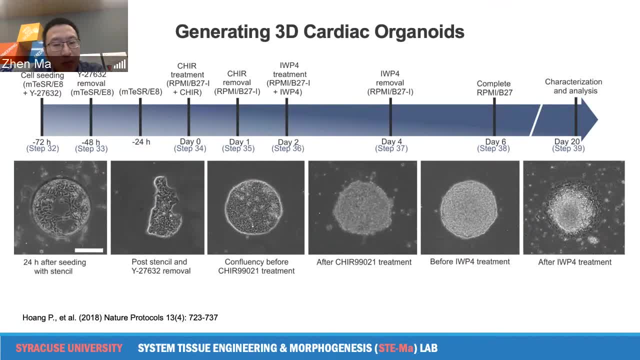 And then we just follow this cardiac differentiation protocol developed by the Sean Palachuk groups using two small molecules to modulate the WIM pathway. The bright field image down below just show you what the pattern cells looks like during the cardiac differentiation. We show this morphology change before and after the TUR treatment and also before and. 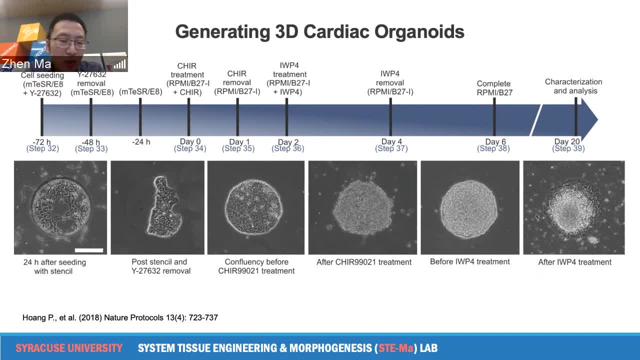 after the IWP4 treatment We start to see the formation of multilayer cell aggregates. after the TUR treatment for the mesoderm induction and the tissue start to condensate to the center after the IWP4 treatment when the differentiation is more towards the cardiac lineage. 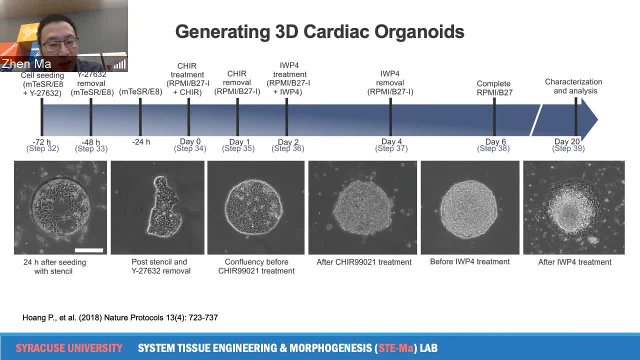 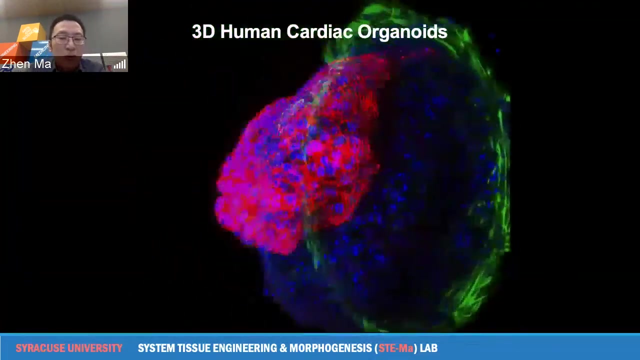 So normally we can have the beating organized starting from day 10, if we consider the different TUR treatments as a day one, and then we run our endpoint merriment on day 20.. So this is our cardiac organize. I like to highlight two things. 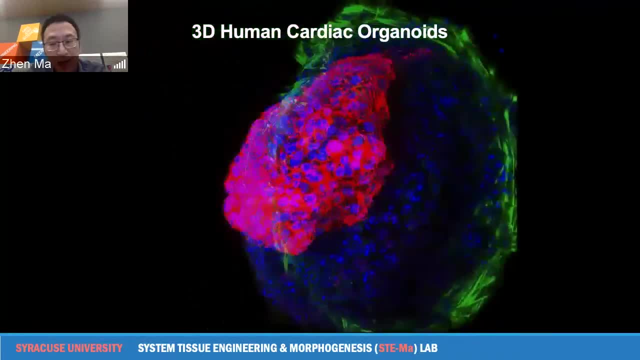 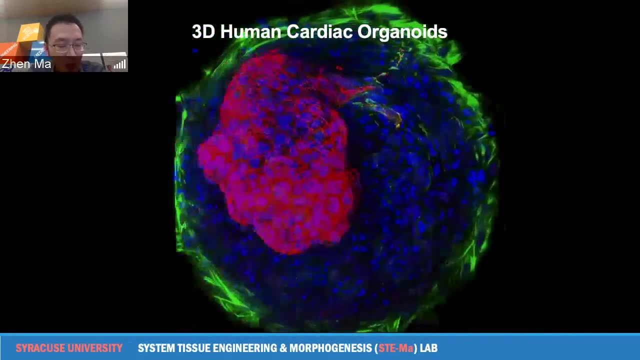 One is our organize. they are generated from two-dimensional iPSCs colonies instead of 3D aggregates that people normally use to generate the TUR, And the other thing that I like to highlight is that they are generated from two-dimensional iPSCs colonies. 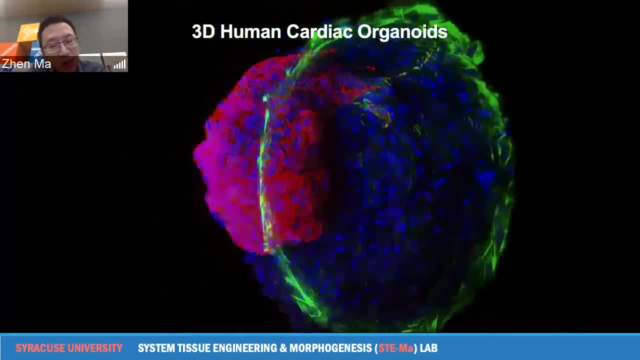 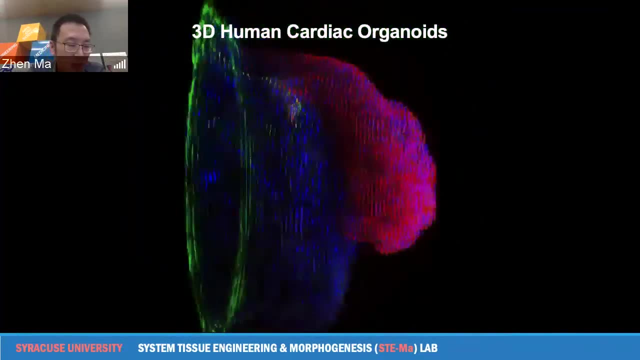 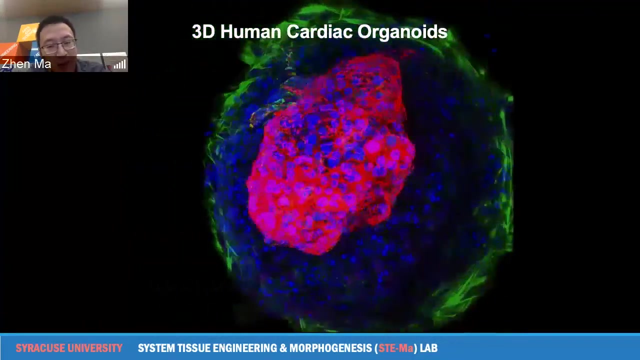 Instead of 3D aggregates that people normally use to generate the TUR, And we think it's a 2D to 3D process that can represent certain level of tissue growth and tissue morphogenesis. The other things we like to highlight is the beating heart muscle is on the center top. 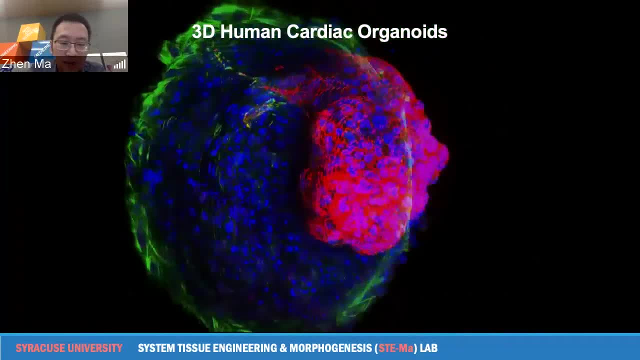 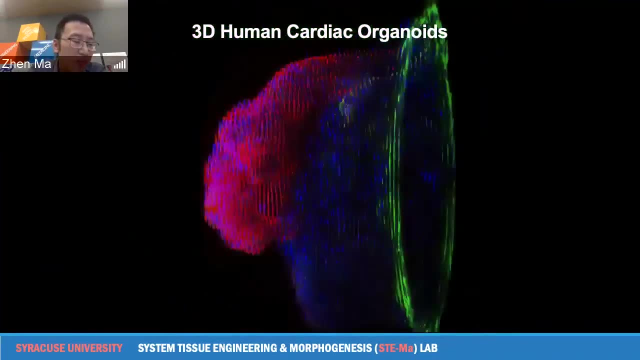 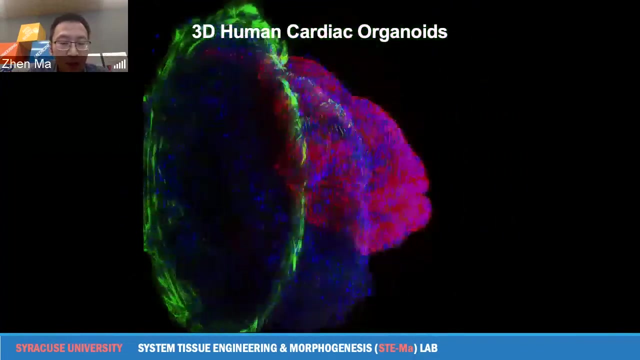 of the organize showing on the red colors but the stromal cells showing as green colors is actually on the perimeter of the organize. It's sort of on the bottom of the organize. This represented the spatial organization of the different cell population within our 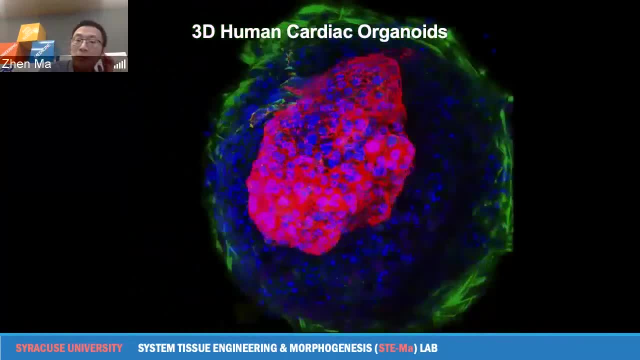 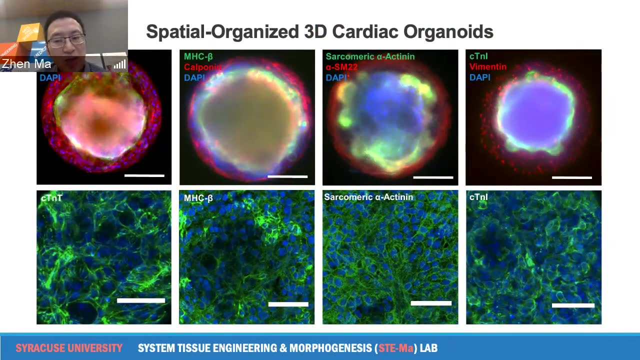 organize. So I will do more staining to show our cardiomyelocytes markers of cardiac triple mu T, triple mu I, myosin, heavy chain, sarcomere, actinine, all these markers indicated by the cardiomyelocytes. it's on the top center. 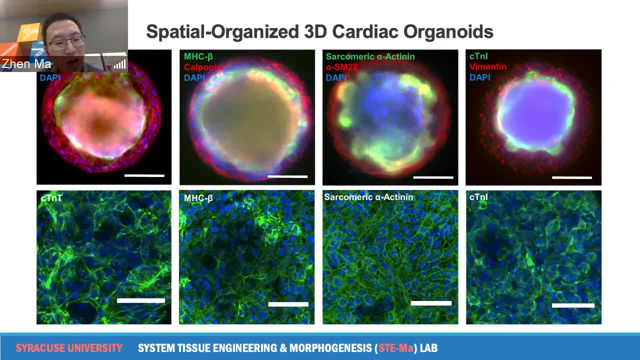 And then we also staining for smooth muscle cell markers of smooth muscle actinine, caponin, XMN22, and vimintin. they are shown more on the outside of the organize. The bottom row of the image are the convocal image of the cardiac markers. 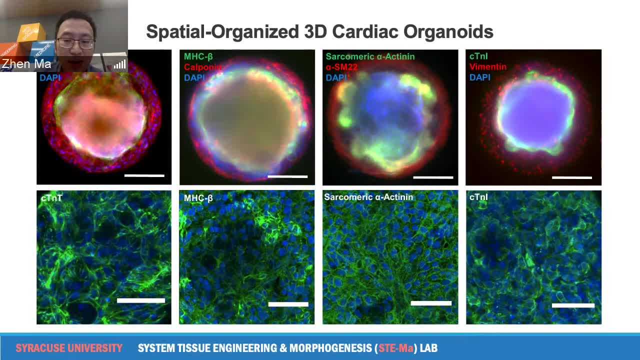 So through this staining you can see the cardiac markers. Okay, So we can see the cardiomyelocytes are not aligned in our organize, which is quite different compared to the other cardiac microtissue study in the field which people try to use. 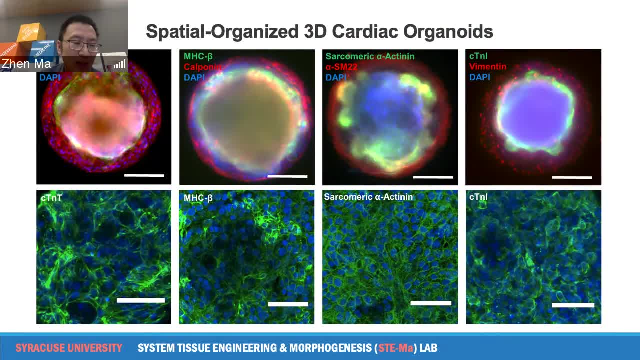 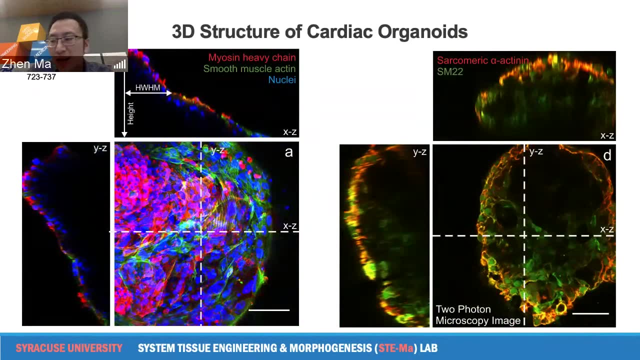 an engineer approach to create this aligned cardiac tissue for more like a physiological relevance functions and the response. Okay, So the image on the left here is a 3D reconstruction of the convocal image of our cardiac organize, which show that sort of a 3D dimensionality of our organize. 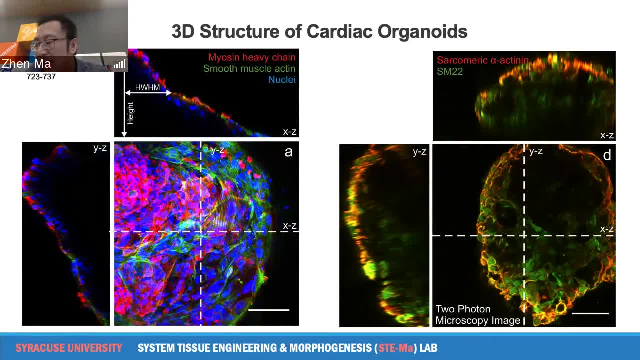 However, you can see there's a huge black- like dark, basically black- region in the center of the organize, And that was because the limitation of a convocal microscopy Okay Okay, So what we're going to do is we're going to go into a 3D image and then we're going. 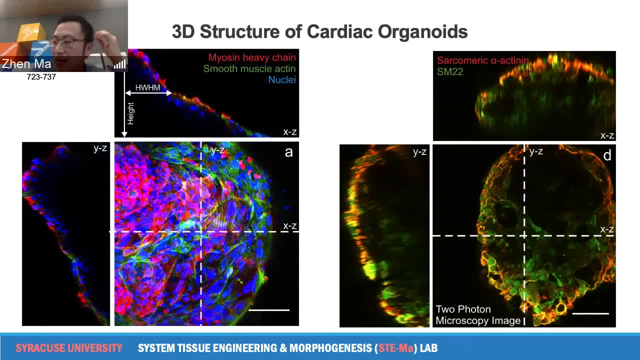 to go into a 3D image And then we're going to go into this 2-fold microscopy which is shown on the right of the slides And you start to see some internal structure of the cardiac organize. We do see some internal region showing there's no cell nuclear indicate that region inside. 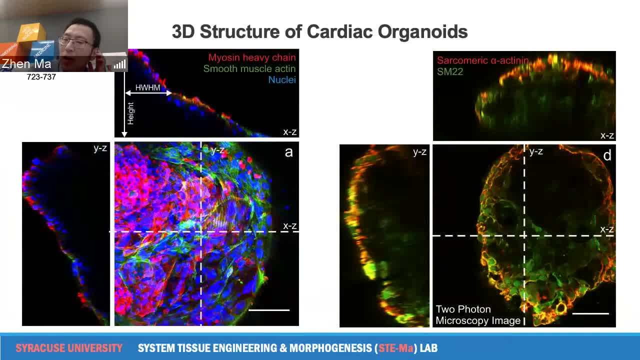 the cardiac organize have no cells. So there's a paper published earlier this year saying people can generate micro chambers in the heart organize. So but however, we don't think we create a true chamber in our organize because if there's a chamber, eventually the organize are going to collapse because all this cardiac 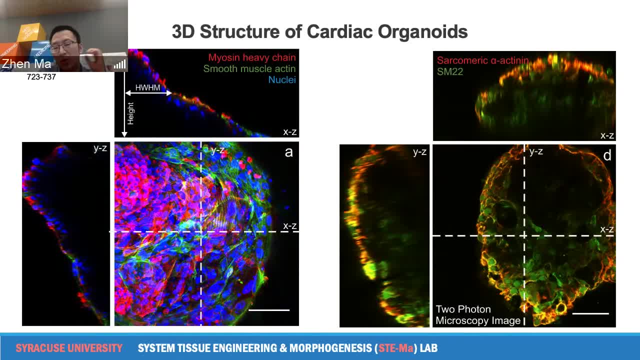 contraction will condensate the tissue into tissue, The tissue into a more like aggregate structures. So we think that the reason we can retain a region with all the cells is because that region maybe was fueled up by the extracellular matrix produced by the supportive cell types. 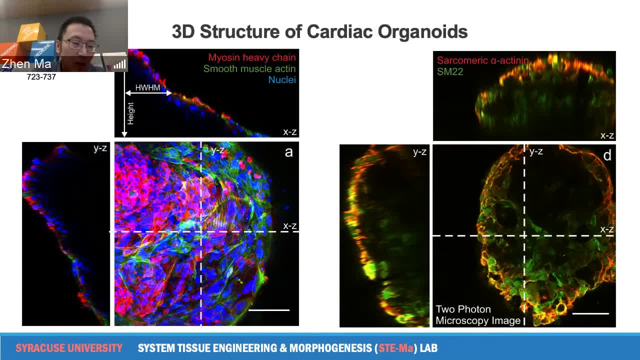 And, like in development, people cause the cardiac jelly so, which is a fuel in the linear heart tube And, I think, something happening in our cardiac organize as well. We haven't really further characterized our extracellular matrix production yet, but that's something we are planning to do. 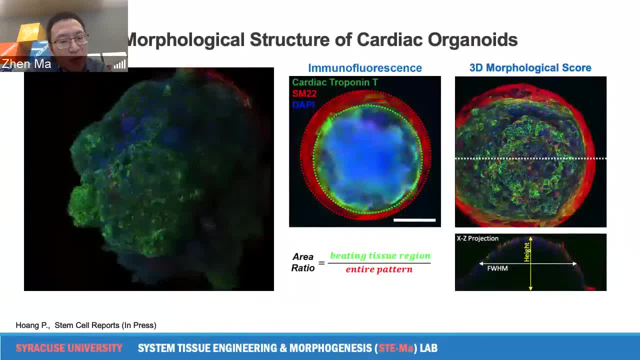 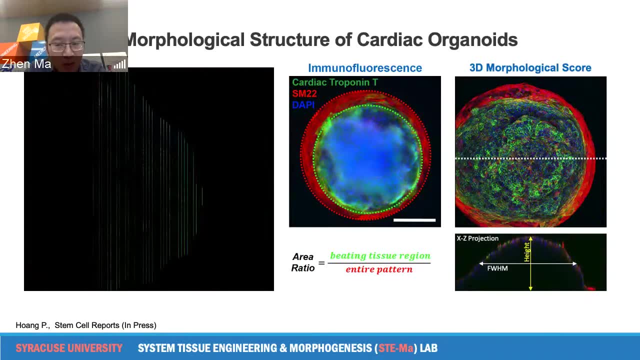 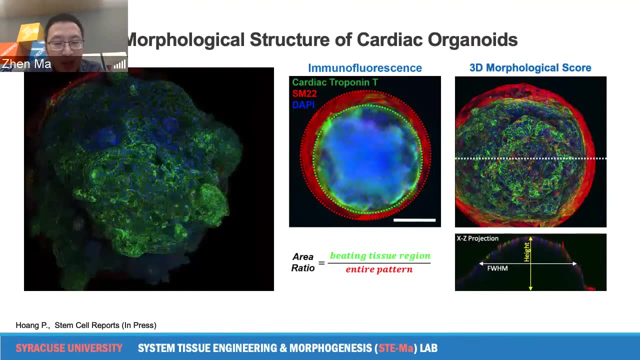 So to characterize the structure of the organize, we can measure the area of the cardiac male side staining and a calculated area ratio between the cardiac male side staining and the cardiac male side staining over the entire pattern size. This can give us an estimate of how well the cardiac differentiation based on the cardiac 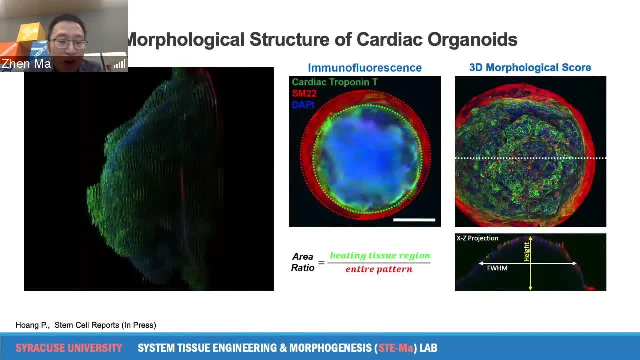 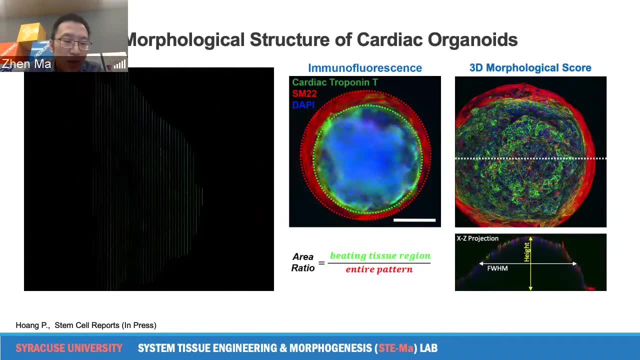 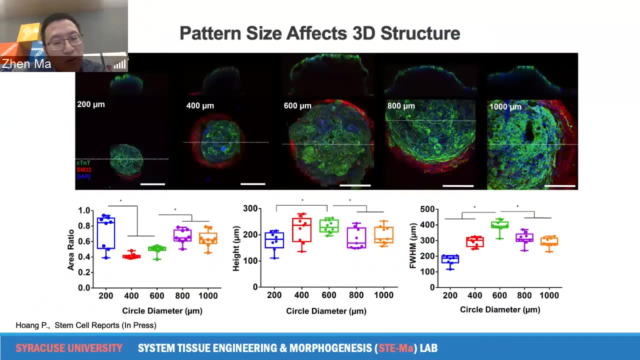 muscle coverage on the organize. We can also measure the height and the width of the organize, which can give us an estimate of how well the tissue grows on the 3D organize formation. So we generate the cardiac organize from circular pattern with different staining. 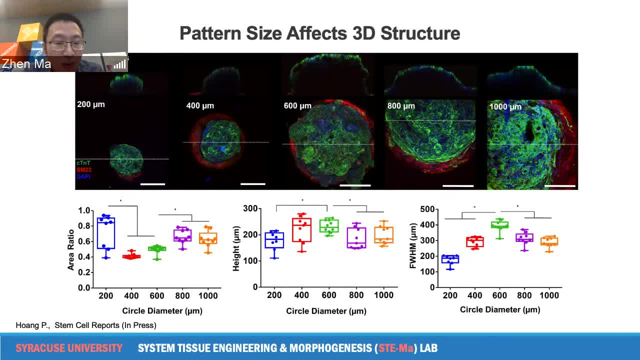 We see from a 200-micron organize showing this high area ratio but much higher data variations. So in general we can now get a consistent organize production from 200-micron patterns And we found the organize from 400 and 600-micron circle patterns have a relative increase in. 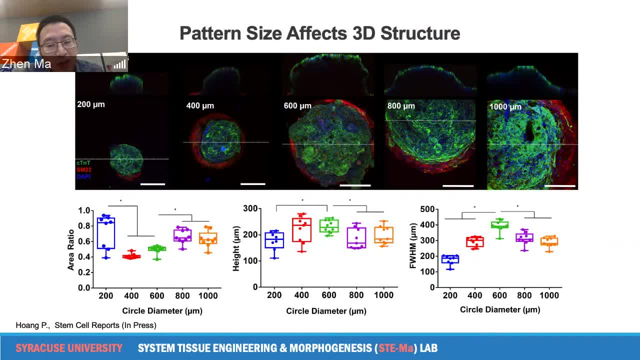 the size of the organize. So we can see that we have a relatively lower area ratio but larger organize height and much better consistency in the organize size and also cardiac differentiations Based on the organize width. we see the organize size are now scaled up with the increase of 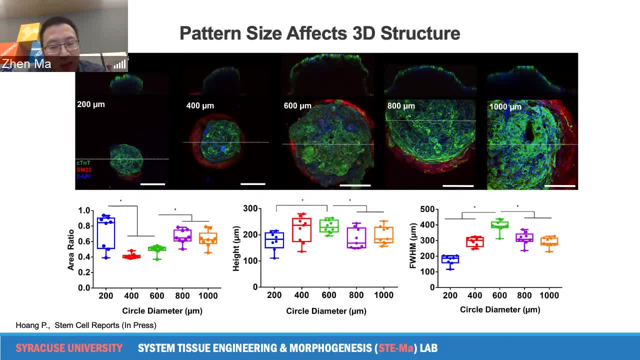 the pattern size. So especially when we move to the larger patterns such as 800 or 1,000-micron, we can see that we have more than 1,000-micron circle patterns. We see the cardiac differentiation have a tendency to follow traditional 2D cardiac differentiations. 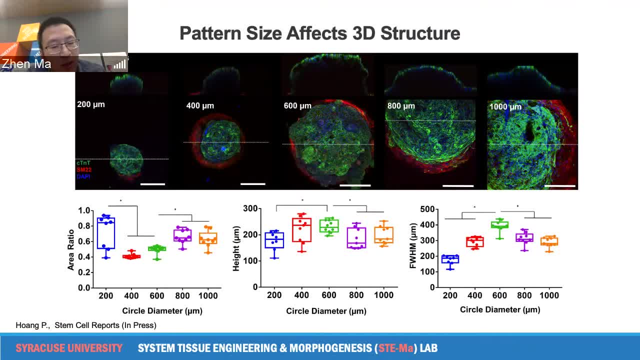 that we see in the tissue culture plate, instead of forming a nice 3D organize structure. So this data tell us a little bit how this initial pattern geometry will affect the three-dimensional structure of the organize and how that will affect the organize productions as well. 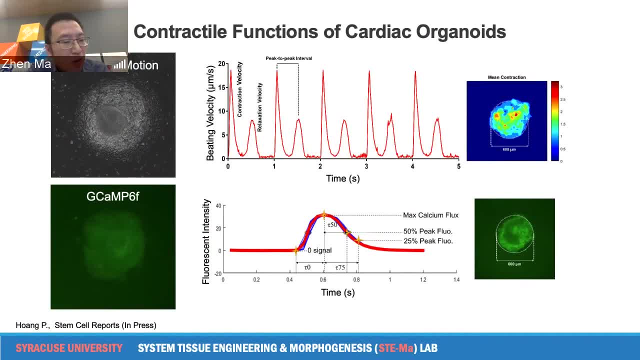 So to characterize the cardiac organize functions, we're using a GCAM reporter iPSL line for calcium handling analysis. So basically we can perform bright field video recording for contractile motion analysis And then we can perform fluorescence video recording for calcium analysis. 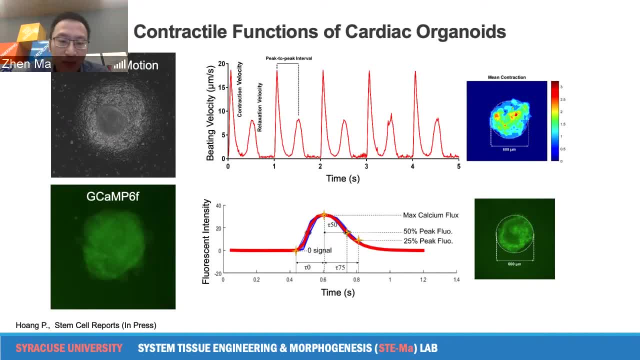 And from this analysis we can extract a series of parameters to quantify the functions which is showing like in this waveform. For example, we can have the parameters of contractile velocities, relaxation velocities, calcium decay time, And then we can have the parameters of short-term, long-term and short-term. 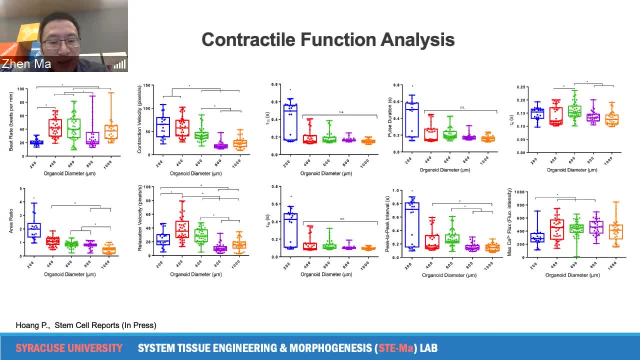 So this is the. So this is a busy slides. I'm not going to like explain this to you. You know why I'm not going to explain this to you in the next couple of slides, But the idea is to analyze so many variables. 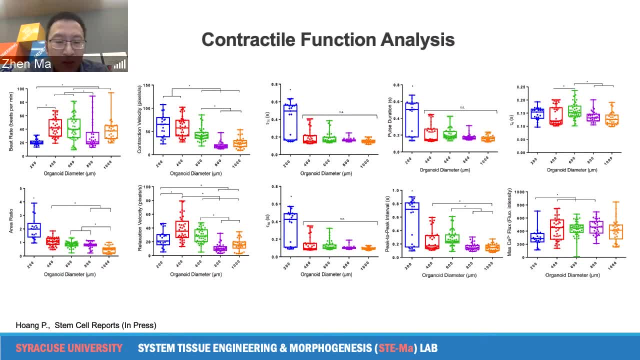 it's hard to make a conclusion. You compare so many different variables for different organoids with different size. it's just hard to extract useful information. So since I started my lab at SU, I started to ask the questions how we can better interpret this data. 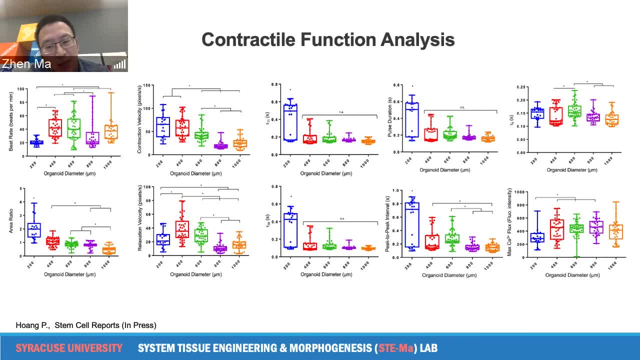 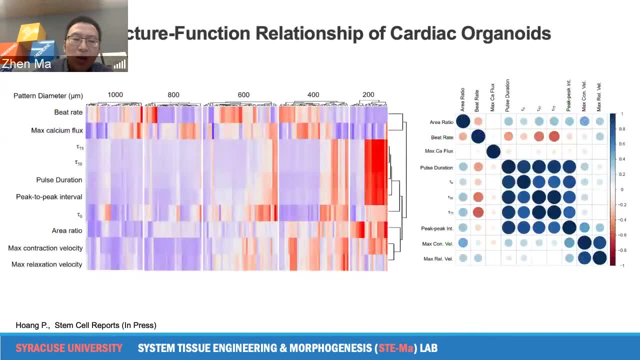 how we can explain this data and what's the key information that is buried in all these different graphs. So what we want to do is to have a better way to analyze and visualize the data using some of the once tools in data mining and data analytics. 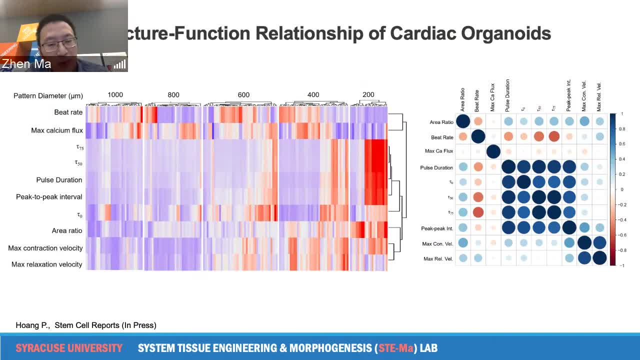 So in this last we put together these parameters for organoids generated from different pattern sizes in this key map And we also show 10 different parameters we can analyze in this data analytics approach. So we further analyze how these parameters can correlate with each other. 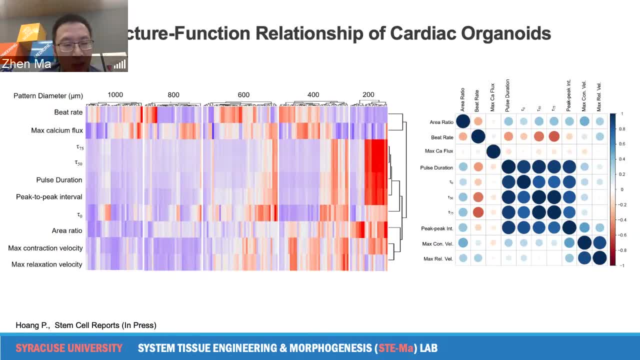 So we can generate this correlation matrix. For example, from this correlation matrix we can see there's a high correlation between this pulse duration from causing analysis and the peak-peak, the interval of contractile motion analysis. which means, if we perform, 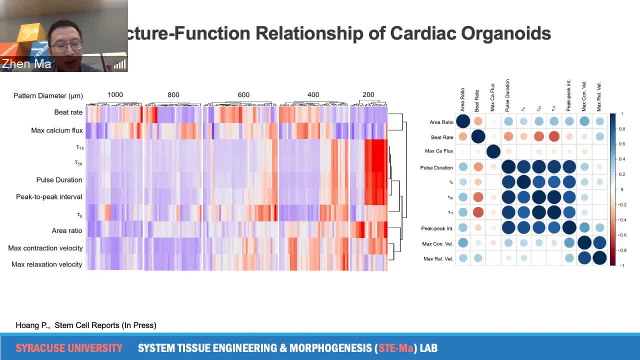 even though we perform two different analysis, the data can highly correlate to each other. We observe this. we also observe that there's a B rate is a negative correlate to the B duration and the causing decay. We also find there's the error ratio. 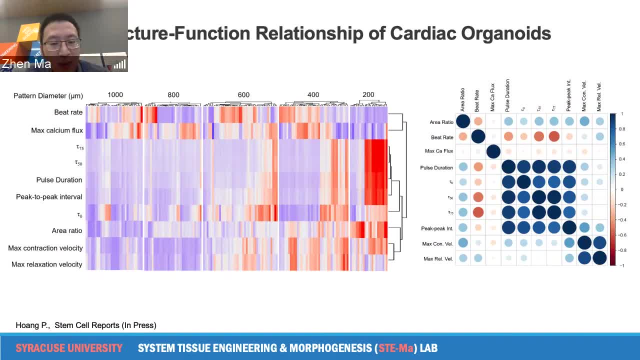 of the organoid morphological analysis is a positive correlate with the contractile motion analysis, which indicate that the larger organoids contract stronger. So basically, using this correlation matrix can help us to establish this structure and the function correlations for our cardio organoids. 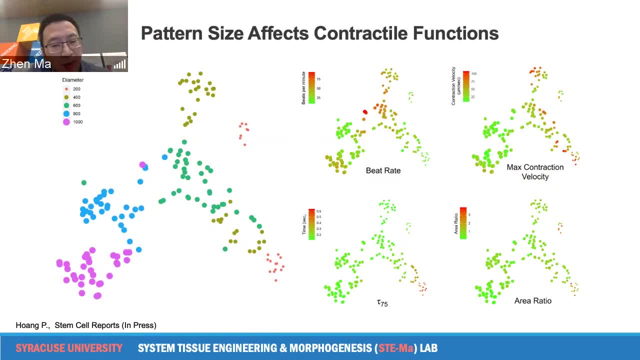 And next we want to see whether we can integrate all these parameters for each organoids, for each organoids. So let's go ahead and analyze the correlation among different organoids. So we're using this t-SNE plot to map all the organoids. 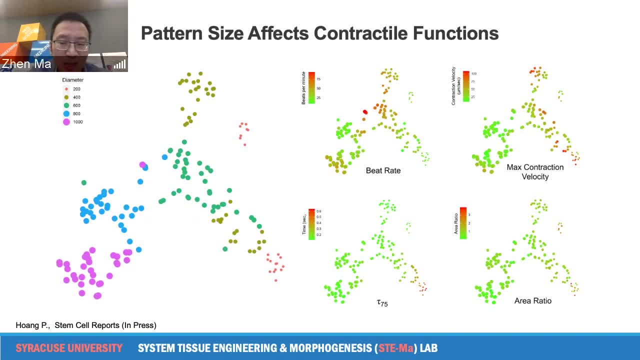 we have collected data from. So basically you can see each dot showing in this map is one organoids integrate with 10 different measurements from period slice. So we observe that the larger organoids from 800 or 1000 micron patterns. they are clustered quite well in the t-SNE plot. 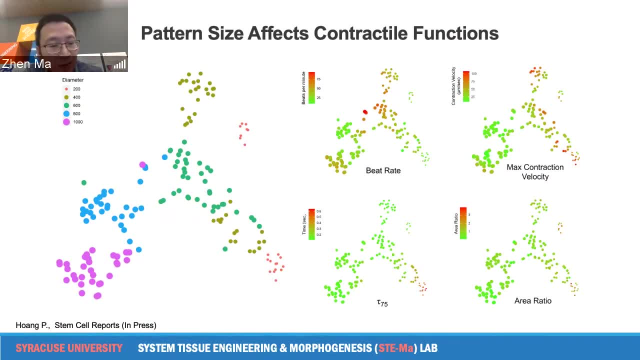 The smaller organoids with 200 and 400 microns pattern size showing there is a separation in the t-SNE plot, which indicate that a larger variation in the organoids functionality for the organoids with the smaller size, The further dive into each parameters. 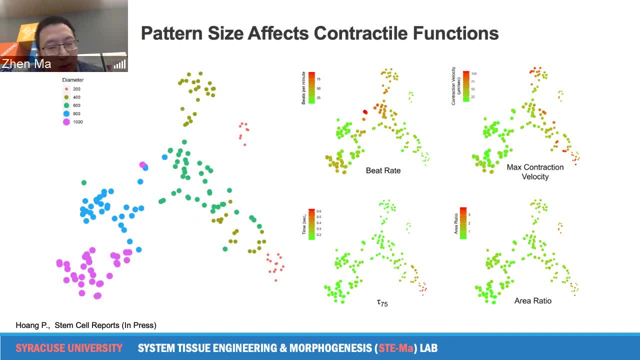 we can see that there's a divergency of smaller organoids is mainly a result from the different. The further dive into each parameters, we can see that there's a divergency of smaller organoids is mainly a result from the different: the difference of the bead duration and the causing decay. 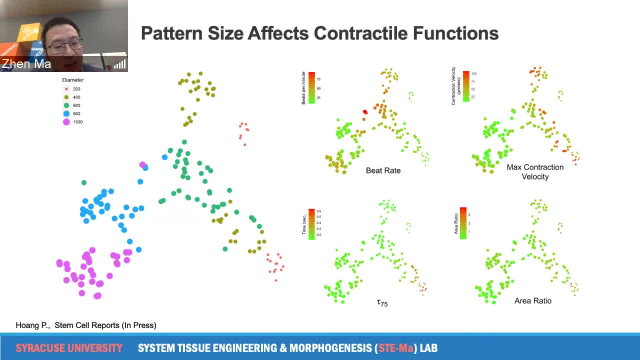 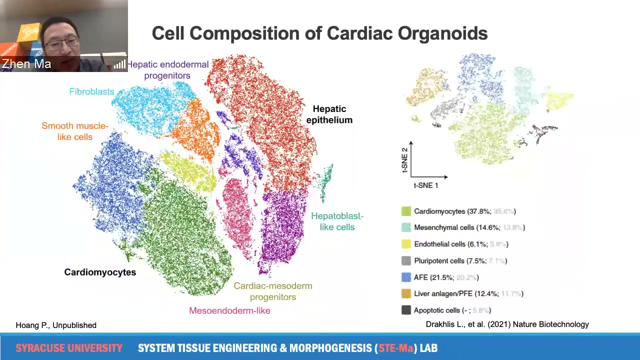 So this analysis can help us to pin down the fundamental key difference between smaller organoids and the larger organoids, which can help us to further optimize organoid productions with consistent functionalities. So, and then to further determine the cell composition of our organoids, we run the single cell RN sequencing. 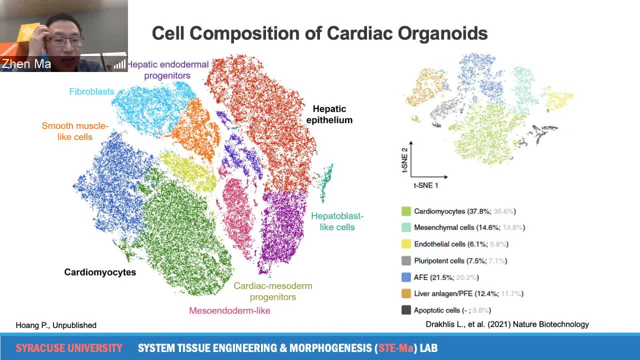 on day 20 organoids and, as expect, we found our cardiomyocyte populations and the stromal cell populations, containing both the fibroblasts and the smooth muscle cells, And, surprisingly, we found a lot of good results in the large population of cells. 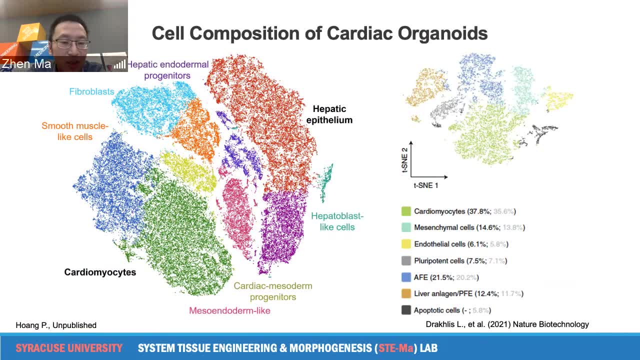 that actually came in from endoderm, showing signature genes related to gut epithelial development and going to early hepatic lineage for liver development. So and this is like we are quite exciting, exciting with our new results. And then we see this publication came out in last month. 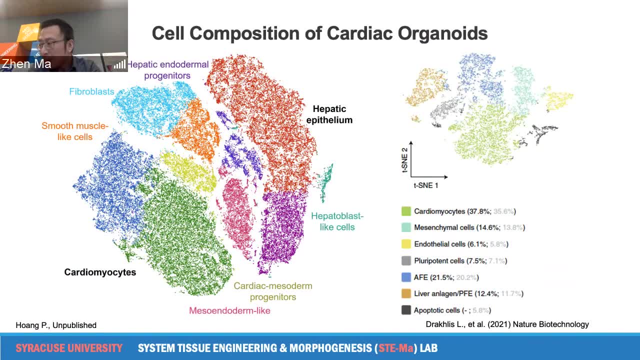 in the Nature Biotechnology They also showed these hard-forming organoids having this endodermal foregut lineage differentiations. So basically they claimed in the the cartilaginous organoids differentiations. the differential protocol will try both the cardiac mesoderm and the cardiomyocyte differentiations. 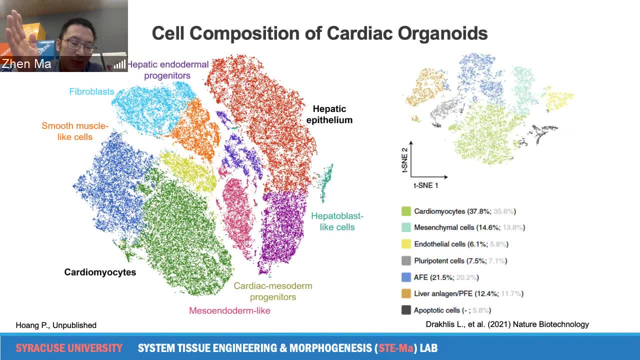 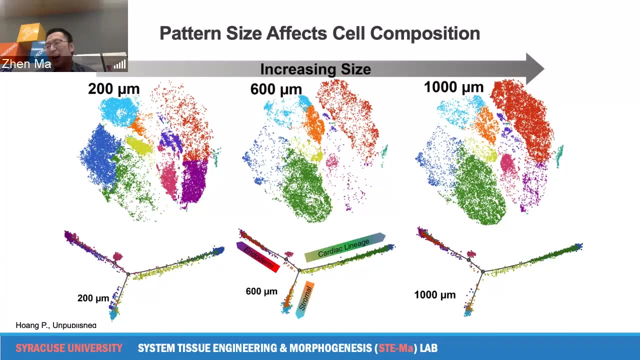 And at the same time the foregut differentiation into both the and the cardiomyocyte differentiation into the different organoids. So these are very interesting into both lung and the liver images. Oh, we are frustrated a little bit by somebody published the data before us. 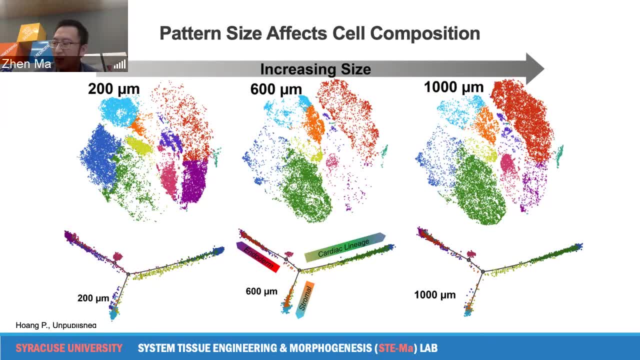 but then we like, we find that there's a new data from our single cell RNA sequencing experiments showing that by changing the geometry of the patterns we actually can tune the cell compositions. Showing this graph we see with a 200 microns patterns: 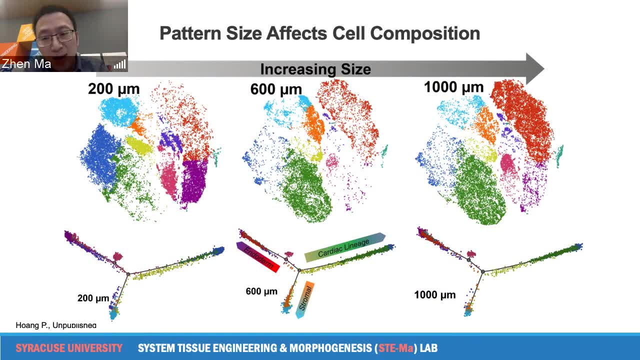 we can generate the cardiac organoids with more stromal cell populations but with the larger organoids from 1000 microns patterns shows a more favorable differentiation into the gut lineage And this middle size organoids with 600 microns patterns actually show a primarily cardiac populations. 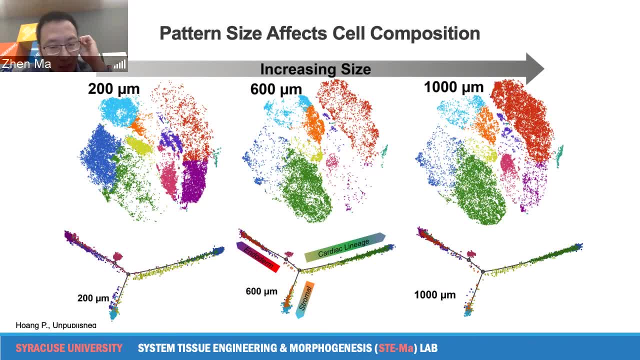 So like one thing I like to highlight here is for the cardiac populations. basically looking at this cardiac mouse size populations, there are actually two separated clusters of cardiac mouse size, showing in the 200 microns organoids as a blue colors, but in the 600 and 1000 microns organoids 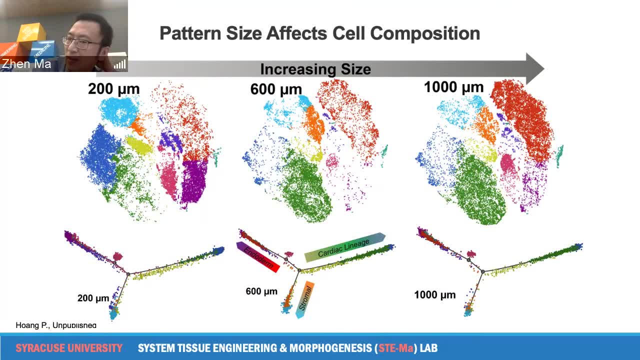 showing us a green colors, which indicates that the different pattern size will change the phenotype of the cardiac mouse size, or maybe a different pattern size will induce the different maturity of the cardiac mouse size. So this is like a slice of our ongoing work. 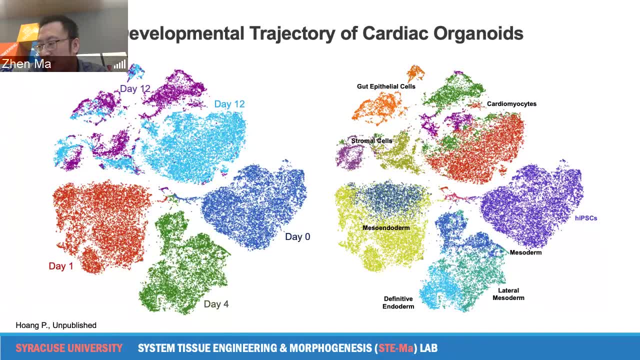 so basically we're just taking the organoids at the different days during the different stations. For example, day zero it's just IPICs, day one is after treatment, after the mesoderm abductions. So basically we are trying to mapping all the cell types. 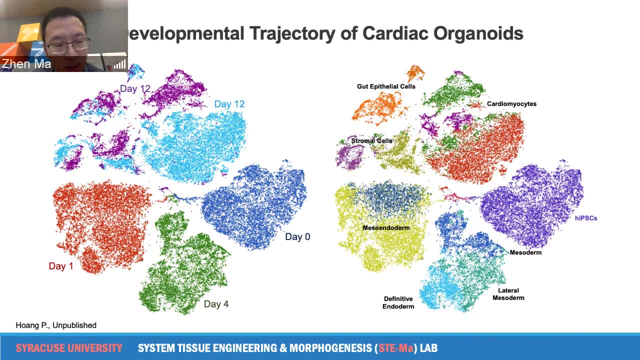 we can find during the entire organoid productions process, And showing on the right is the different cell types. We are still need to further dive into development biologies, And then we also establish a new collaboration with Ben Cosgrove lab at Cornell universities. 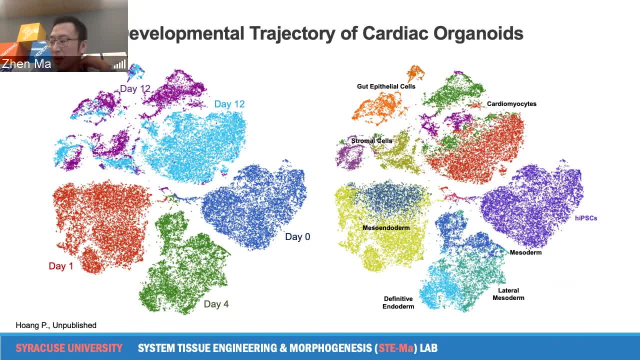 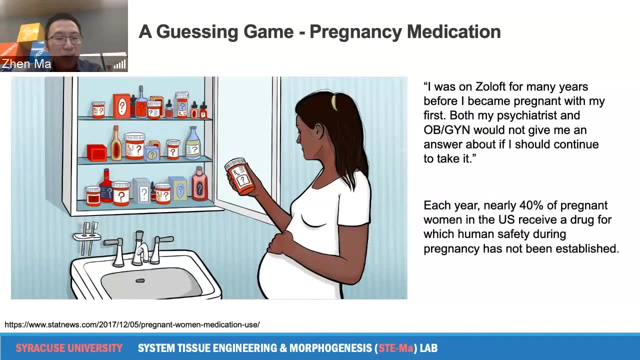 and try to use them. There are more advanced bioinformatics tools to help us to see more subtypes, cell populations, in our single-cell RNA-seq data. So now I'm gonna switch gear a little bit and talk about the application aspect of our organoid model. 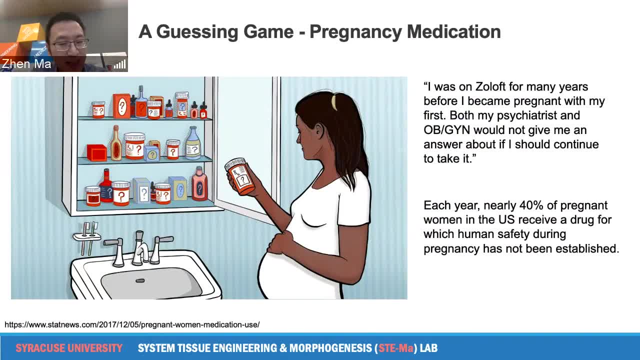 So taking drugs from pregnancy is always a guessing game because we are so afraid that the drugs will have side effect that will influence the healthy fetal development. However, nearly 40% of pregnant women in the US still receive a drug which the safety for the fetal development. 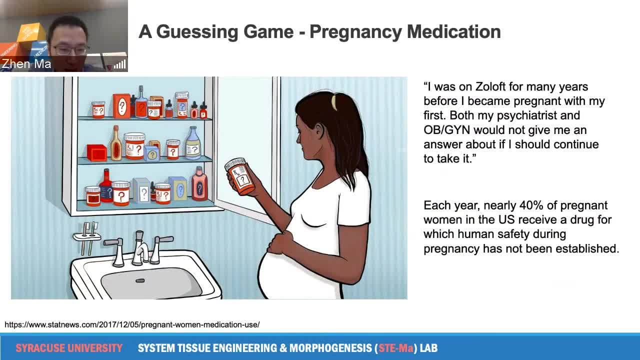 has not been well established yet. So this comes to a very difficult and a crucial decision for the expecting mother about their pregnancy medications, especially for the women who are suffering from mental disease, because of the safety for psychiatry drugs during pregnancy are not well studied and established. 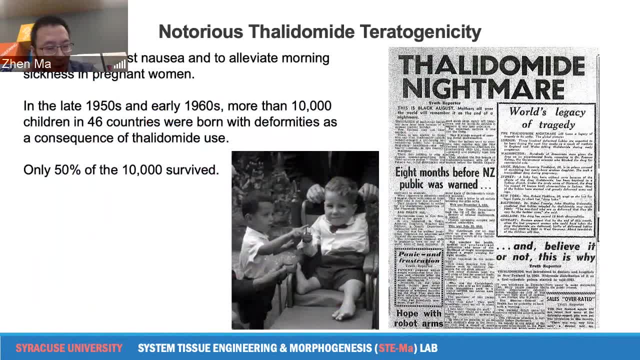 When we talk about this drug- induced teratogenicity- we can now ignore this thalidomide tragedy in the history. So this drug was first developed to treat nausea and then the pregnant women taking it to alleviate the morning sick In the late 1950s and the 1960s. 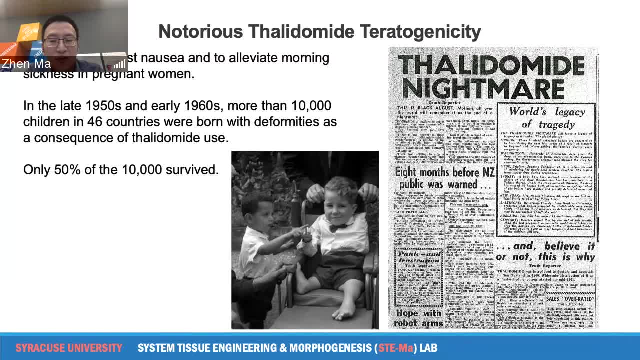 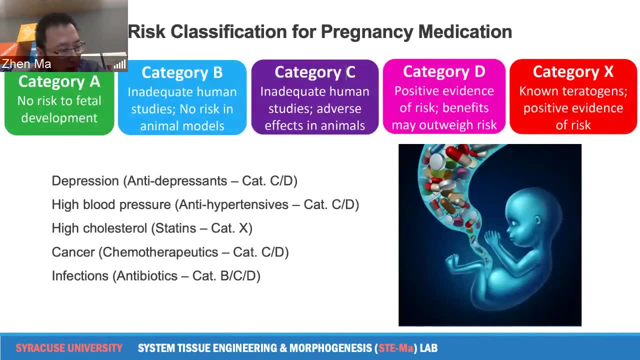 more than 10,000 children in 46 countries were born with deformities as a consequence of thalidomide use, And unfortunately, only 50% of the babies survived. So this tragedy pushed the FDA to establish it as a drug category that can used to regulate. 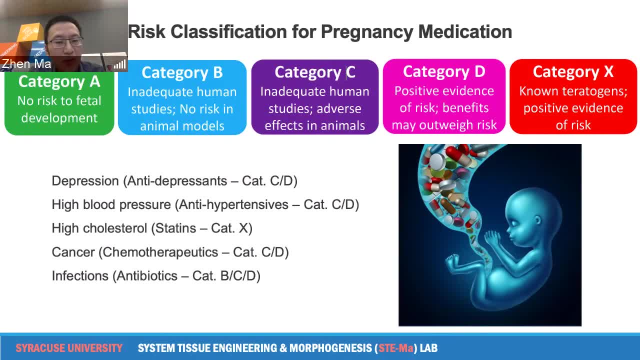 the drug prescriptions for pregnancy women. From the category you can see- any drug from C to X will potentially have adverse effect on fetal development And unfortunately, a lot of drugs we use as an entire health factor, used for treat disease or syndromes, fall in this category. 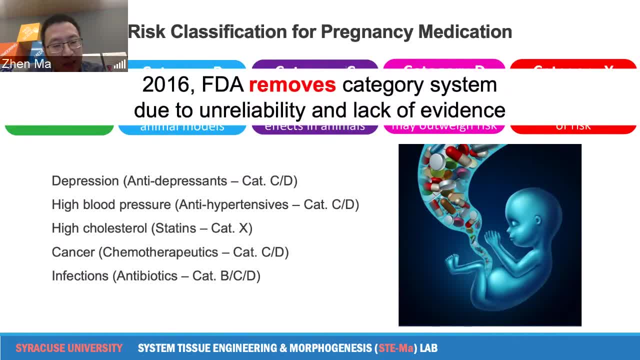 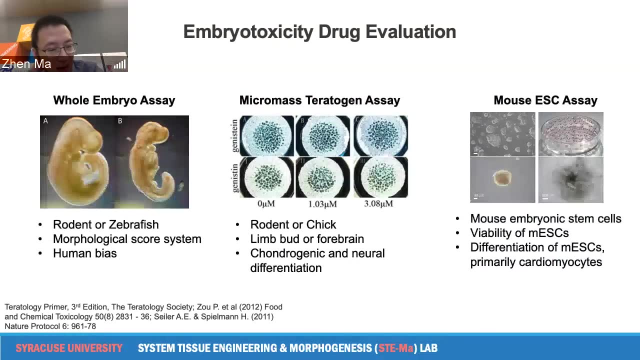 However, in 2016,, FDA decided to remove the drug category system due to unreliability and lack evidence from human related studies. Oh, one major reason of this unreliability came from this assay system that for the embryo toxicity screenings that pharmaceutical company has been used for decades. 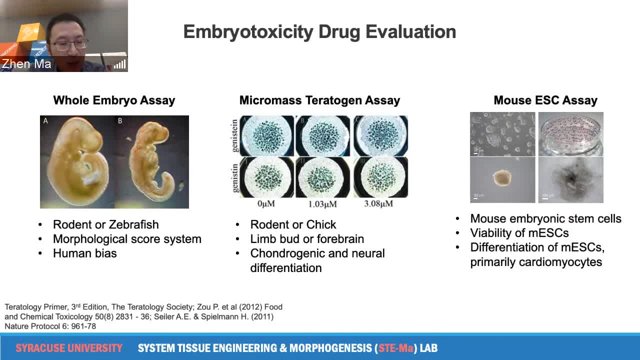 Here's the three assays, including the whole embryo assay based on rodent or zebrafish micro mass assay and the mouse embryonic stem cell assay. There's no human assay available And, more important, only the whole embryo assay. provide us this morphological screening. 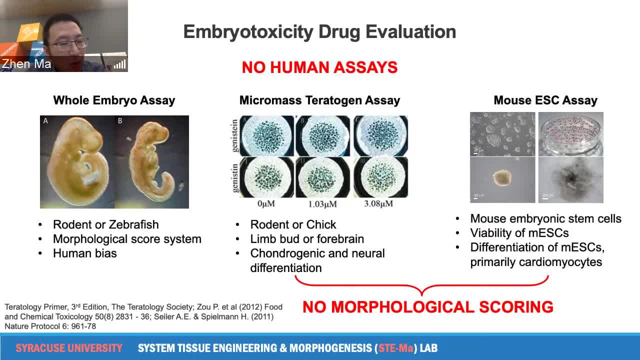 that evaluate whether the tissue or organ can develop into the right form under the drug exposed. So what we really need to establish is to create a human model for embryo toxicity test, which have the capability for morphological scoring Well, taking our advantage off of cardio-organ models. 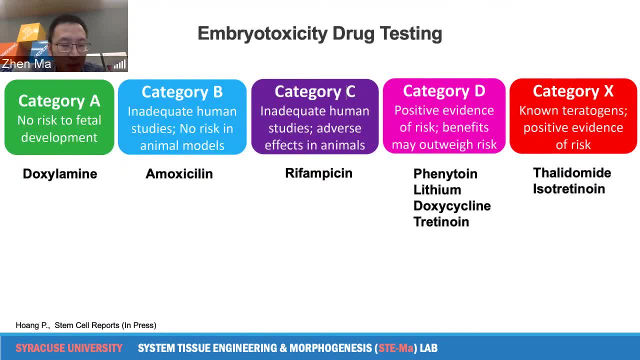 we test many drugs from these different categories with a different potential of the embryo toxicity. Just be simple. you can think with the increase of the category from A to X, the severity of the embryo toxicity level is increased. So for the time I'm not gonna show all the results. 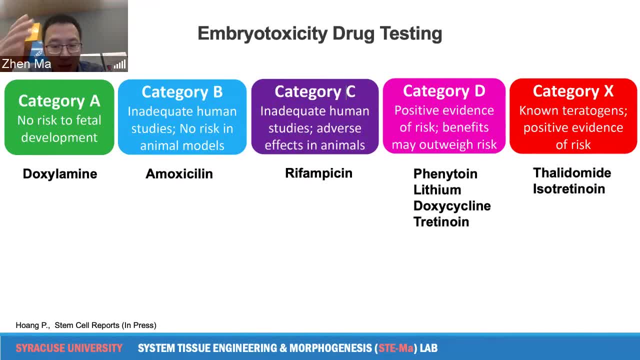 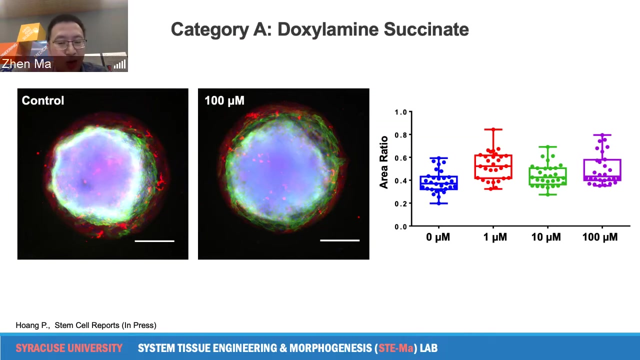 for every single drugs, but in the next, like 15 minutes, I'm gonna try to focus on some key interesting results we observed from our drug screening test. So first we test our category A drug, which means there's no effect on embryo development. 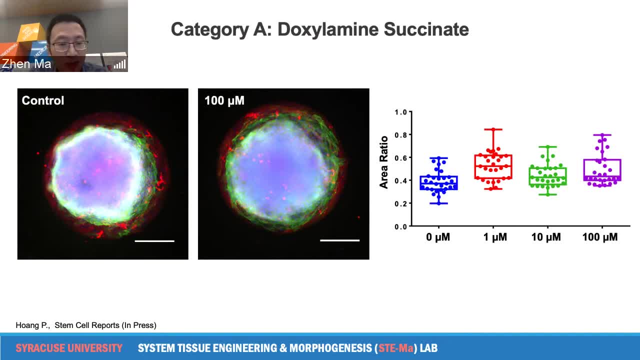 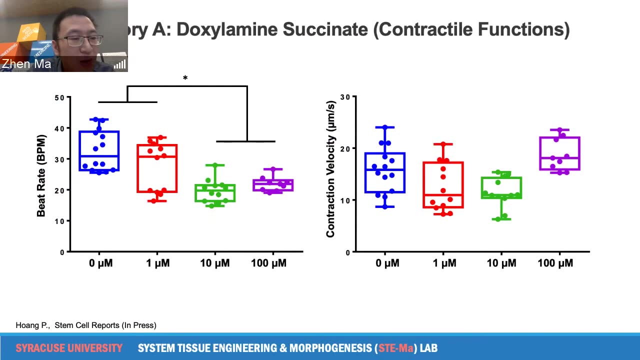 We didn't see any difference on the area ratio across the different dosage on the organoids. So we're gonna test it, And we also. but, however, we do see that the drugs have an effect on the B-rate. One reason: because this drug was prescribed as a sleep aid which can reduce the muscle contractions. 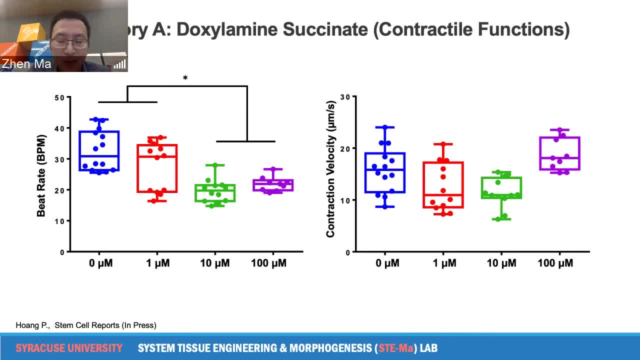 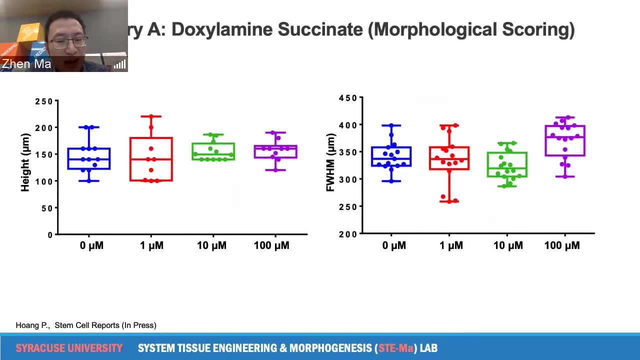 That's the reason we have like a lower heart rate that can help us to go into the sleep, And these drugs do not affect the height or the width of the organoids, indicating that the organoids can grow into the right three-dimensional structures. 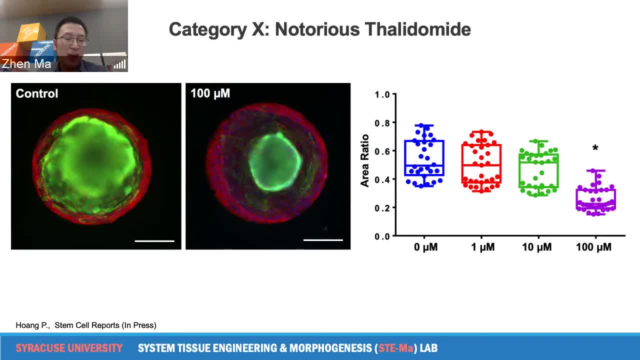 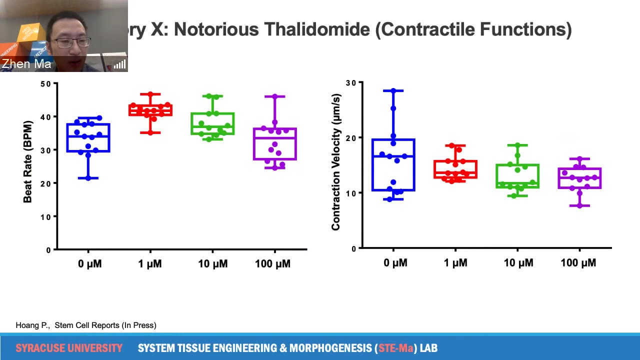 So then go to the total the other way. we test this selenamide, which is a category X drugs. We find this at a high risk dosage. it will significantly diminish the cardiac activity And surprisingly, the selenamide does not affect the contractile functions from the organoids, at least from the motion tracking analysis. 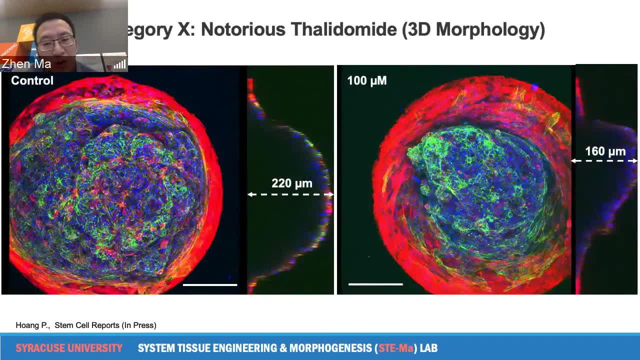 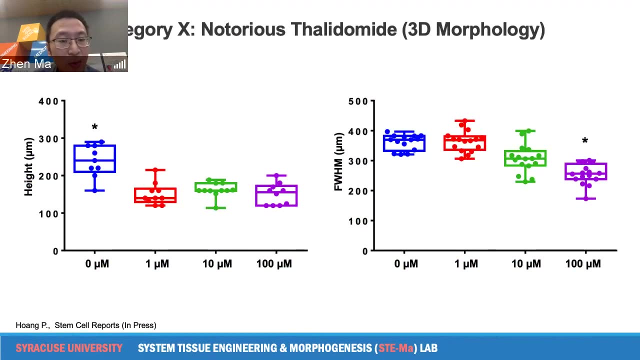 But when we perform the confocal image of the organoids we can see the 3D morphology of the organoids was a significantly impact by the drug, drug exposure. So we found that even at a low dosage and one micromolar, the selenamide could significantly reduce the organoid height and limited organoid developing into the right structure. 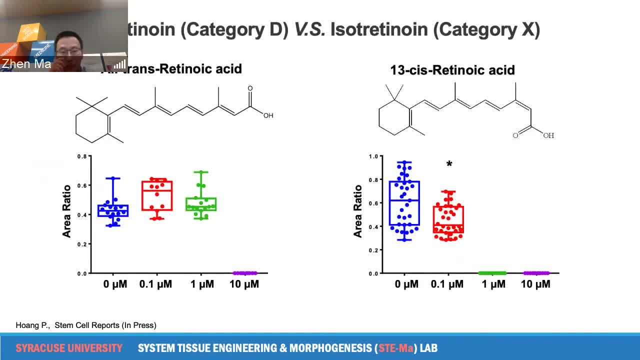 I also like to highlight this drug, this radionic acid. There's a two version of the radionic acid, trinidinoin, And I'm going to show you the two versions of the radionic acid: trinidinoin and radionic acid. 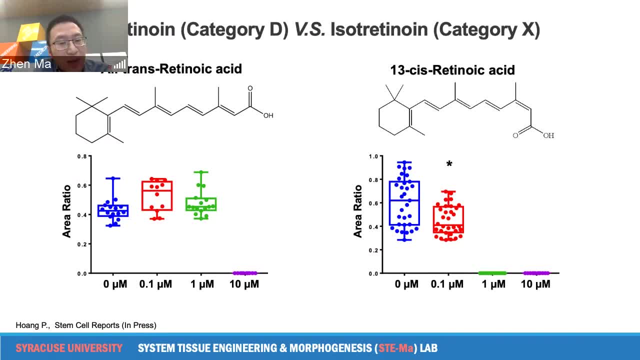 And I'm going to show you the two versions of the radionic acid. The difference is only one chemical bond rotation, which makes one drug as category D and the other one as a category X. So when we test these two drugs using our organoid models, we found that category D drugs with less embryo toxicity can generate the organoids at one micromolar. 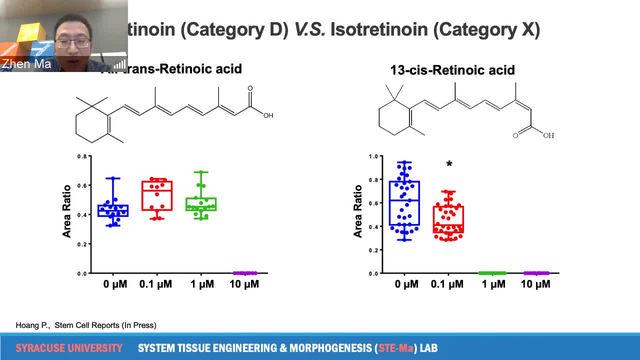 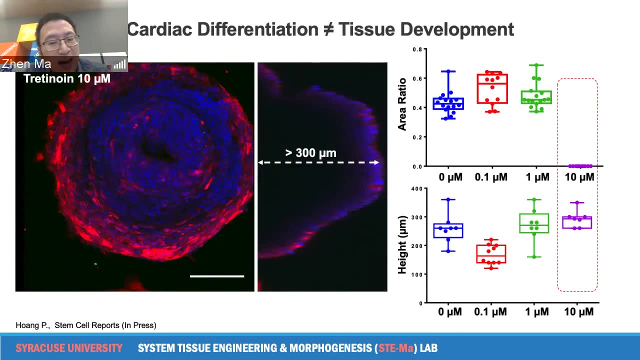 But the category X drugs, again only one, And that's the difference. one chemical bond rotation cannot generate organoids at the same concentration. More interestingly, we know, at the highest dosage of the retinoic acids there's no cardiac differentiation. 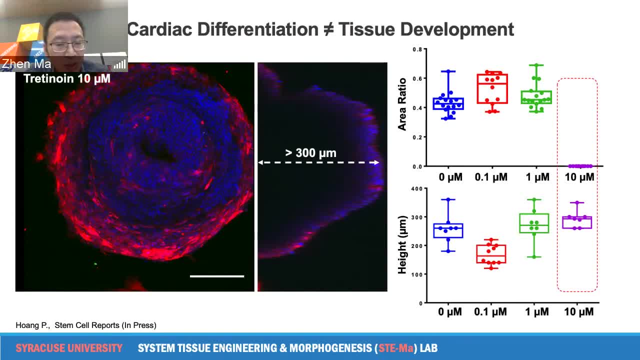 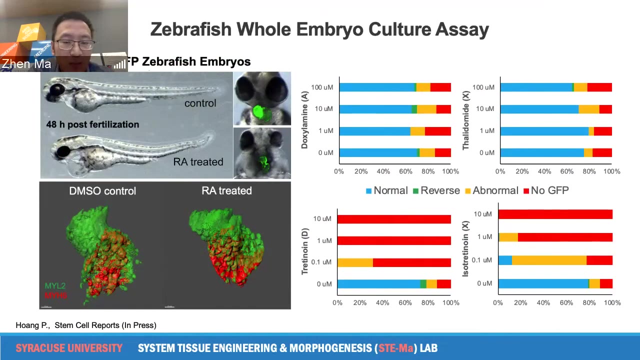 but we still can find a formation of a giant 3D tissue structure which is even larger than the normal cardiac organoids. This told us there's no cardiac differentiation does not mean we cannot get a large organoid tissue formation. So last we also compare our result. 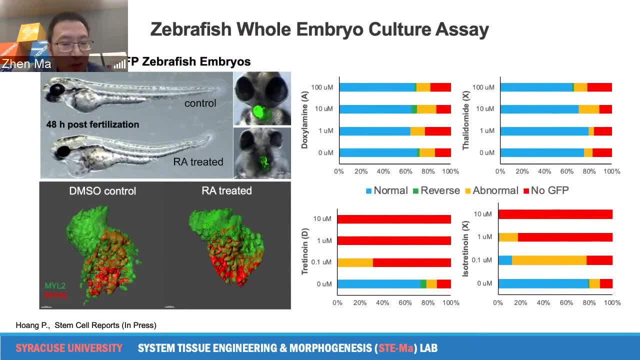 with zebrafish embryo models- This is a transgenic zebrafish model- has reported on a melting light chain So we can analyze how the drug will affect the looping of the heart tube in the zebrafish. For the four drugs I mentioned, 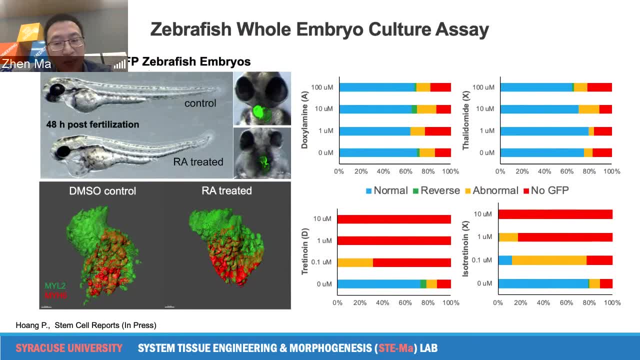 here we found a consistent result of the sleepy eight, that's, the category A drug and the retinoic acid, between the human organoid models and the zebrafish embryo models. However, the selenite exposure did not induce a significant impact on the zebrafish model. 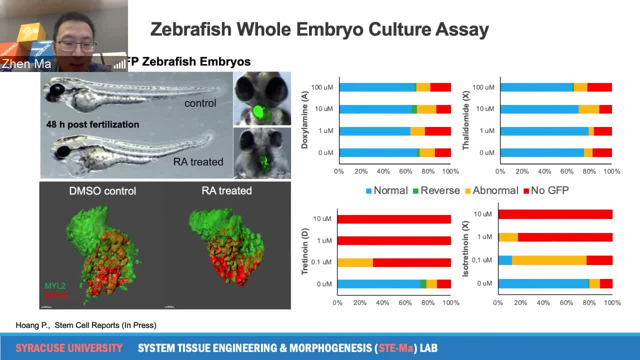 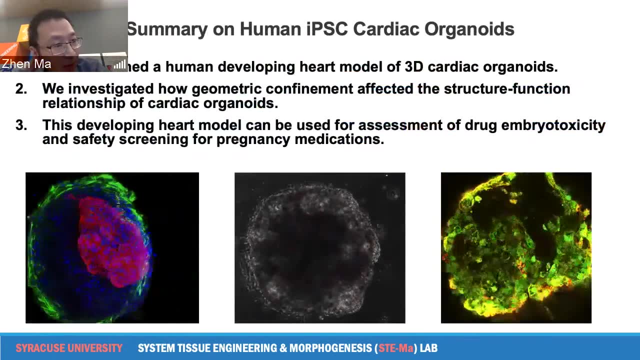 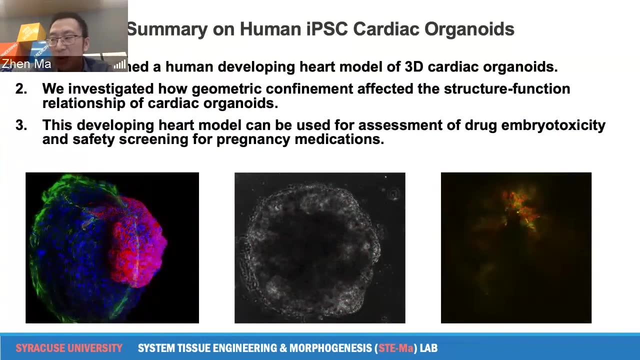 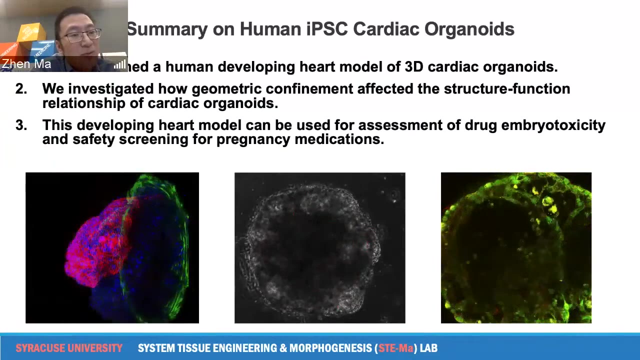 which highlighted the need of a human-based assay for the embryo toxicity. To summarize my talk on the IPI's cardiac organoids, we established a human development heart model. on the cardiac organoids. We investigated how these geometric confinements will affect the structure-function relationship. 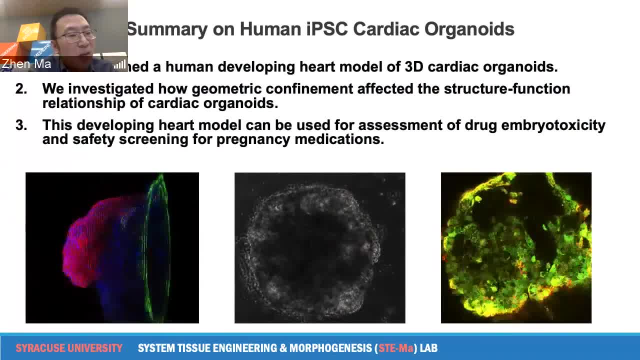 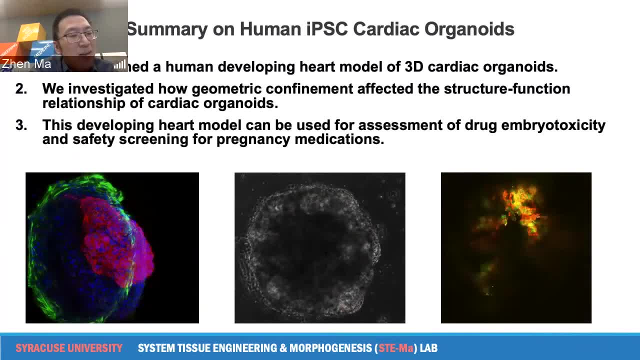 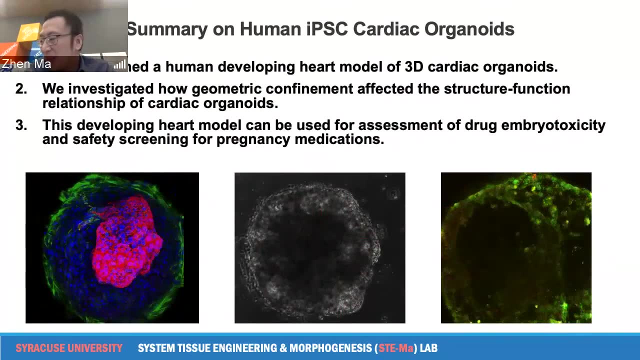 of the cardiac organoids, And this developing heart model can be used for the assessment of the drug embryo toxicity and the safety screening for pregnancy medications. So I think I'll just stop here. I don't think I have time for the mesenchymal stem cell part. 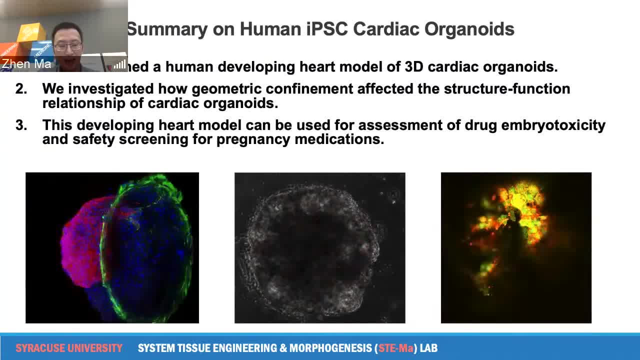 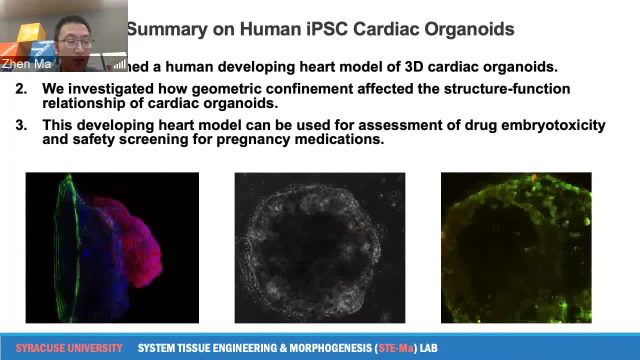 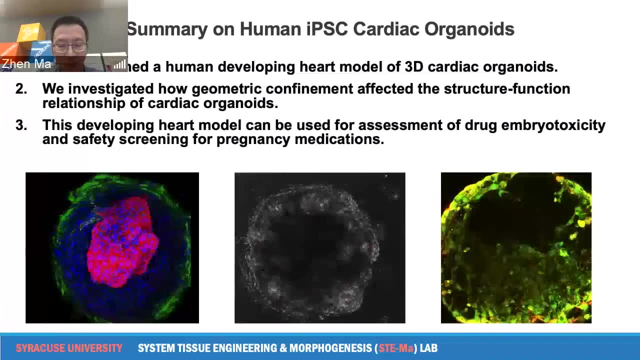 I can take questions And, for the people interested in the mesenchymal stem cells, we differentiate in the lab. we can talk more in our meetings or, if we don't get to meet, you can just send me an email If you're interested in the mesenchymal stem cell. 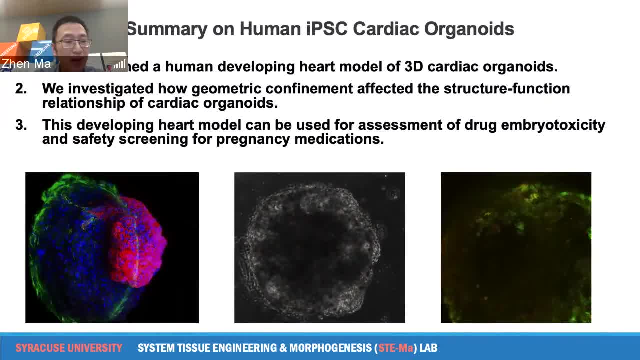 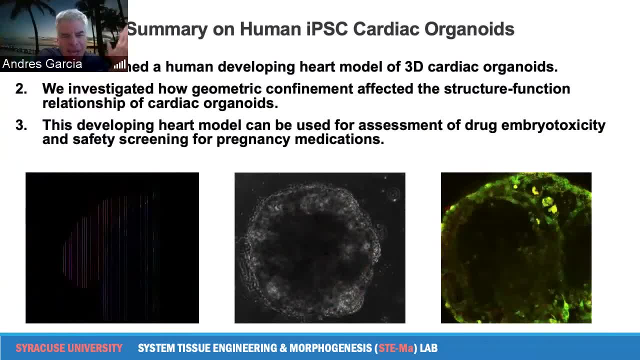 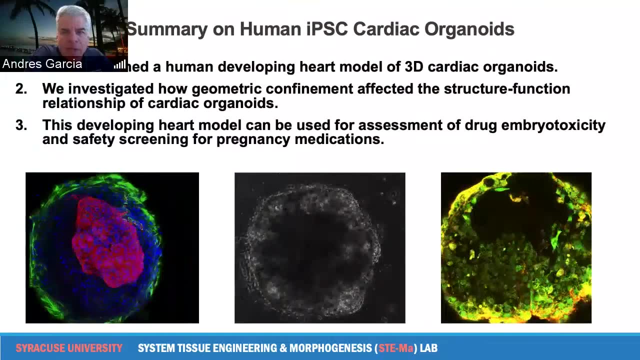 that we can differentiate from human IPICs, And thank you very much for your attention. I'm happy to take questions. Great So, virtual clap. Thank you very much. That was a great seminar. Please post your questions in the chat. 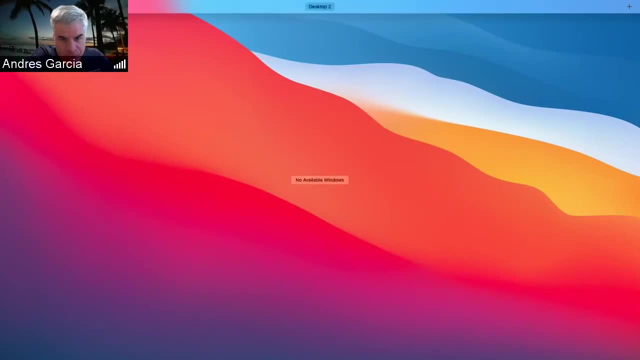 Chen. we have three questions, so I'll go through those. Okay, So the first question is: do you have any questions? The first question is from Professor Mantellaris: Could the higher variability observed in the 800 to 100 micron organoids? 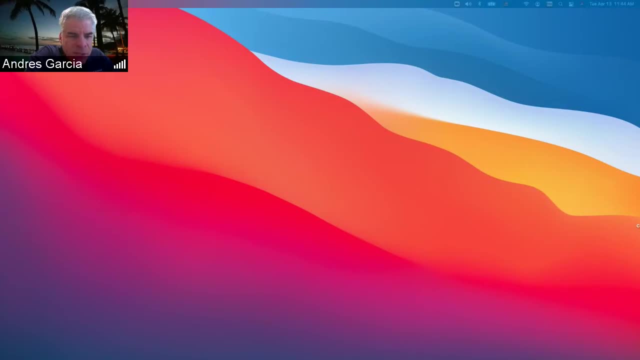 be due to potential mass transport limitation. I think he's referring to the first part of your presentation. Yes, yes, So data variations we see like among the organoids, right, like, especially when we do this t-SNE plot and try to see how all the organoids can cluster each other. 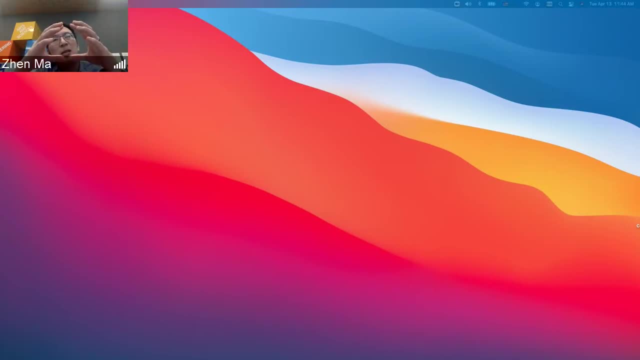 We see in most cases the larger pattern, size, the organoids. they can cluster quite well in the t-SNE plot which means there's a higher, more consistency in the larger organoids compared to the smaller organoids. And so I think like if we couple, the functions result. 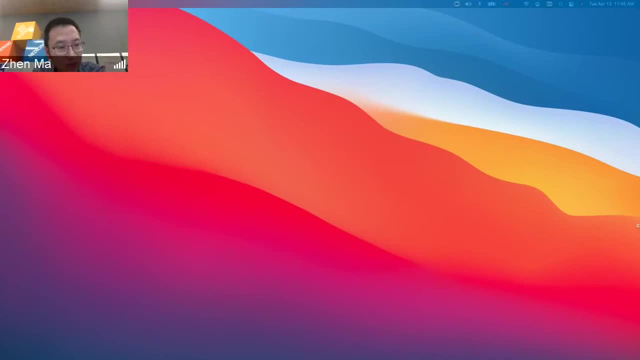 with the single-cell ion sequencing result. like from the single-cell ion sequencing result, we show there's a more progenitor cells and the stromal cells are located in the smaller organoids, which means the smaller organoids, either in the phase. 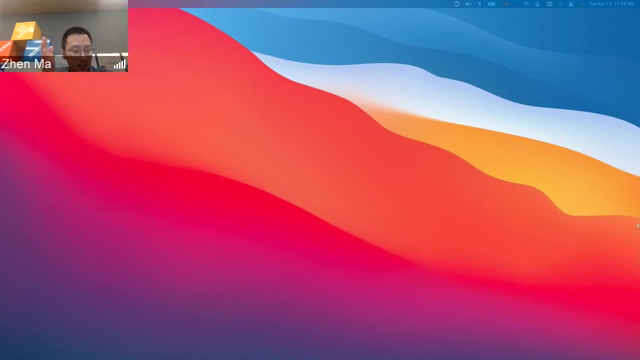 which now fully differentiate, at least at the day 20 mark, or they are locked in the stage. they can now fully differentiate into end, fully differentiate the cardiomyocytes or the gallium And I think that like a progenitor stage. 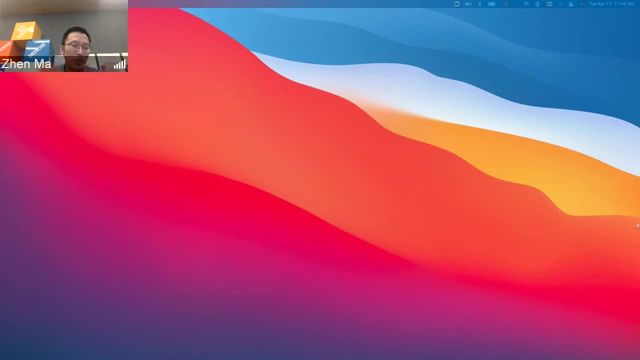 we'll create a lot of like variations in the functionalities that we can measure it in the endpoint measurements. So, And I was gonna say Saki's followed up with a sort of a more general question: Mm-hmm, What is the influence? 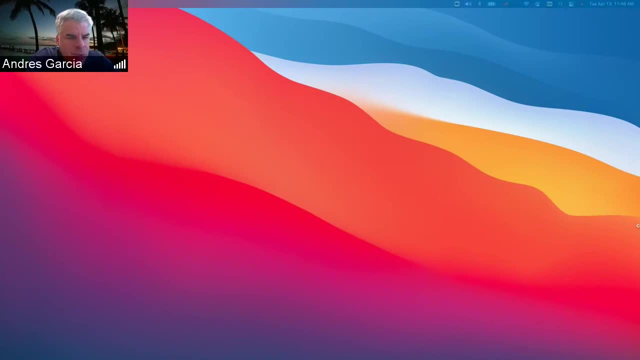 of mass transport in the results Because you have this very large cell aggregates, right. So you think about like the organized, more like a dome shape, right, And our organized never really go above 300 microns. So if you think about, the core is the center. 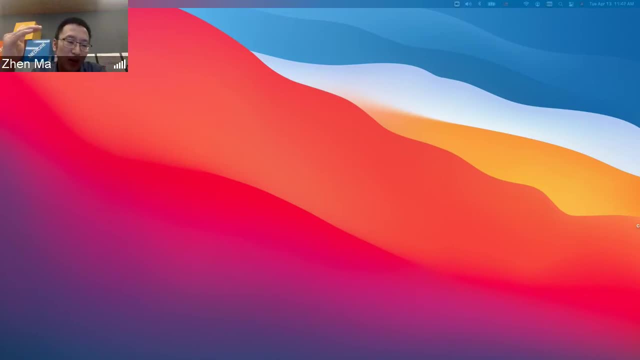 it's never really sort of reached the limits of the nutrient penetration, about like 200 microns nutrient penetrations, right. So one thing I think that you cannot development even longer or larger is because the limitation of the nutrient transport. So there's only a couple of cases we see. 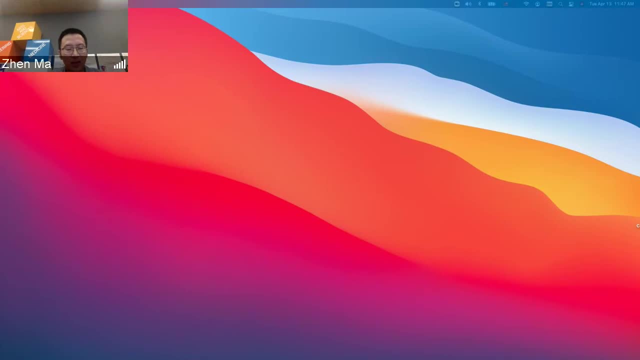 that they can grow a huge like organized. that actually from our radionic acid treatment we don't really. we cannot really see inside yet. but maybe there's a necrotic core developing the center of in the organized. we cannot just see. 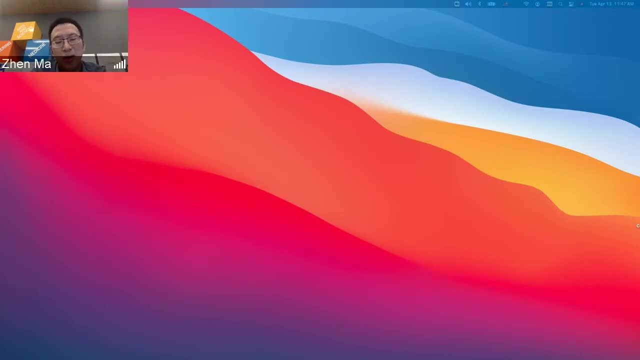 So for like smaller organized, I don't think there's a nutrient transport issue occurs. Okay, thank you. Okay, so we have a question from Hannah Song. 3D cardiac organoid generation looks very interesting In the heart cardiomyocytes and cardiac fibroblasts. 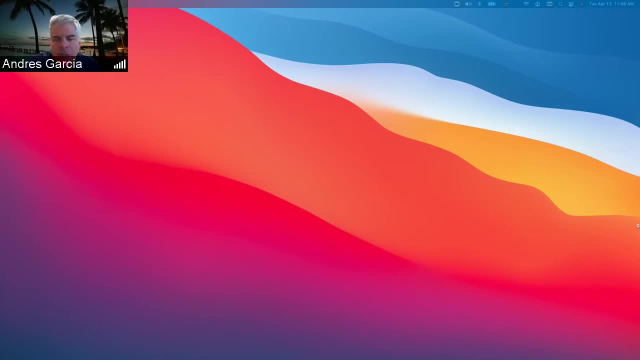 arrange almost like alternating each other In the organoid. it seems like they differentiate and proliferate separately. Any idea what kind of signaling is involved in this? two different development like processes? Oh, we haven't really looked going to the signaling part, but I can tell you literally: 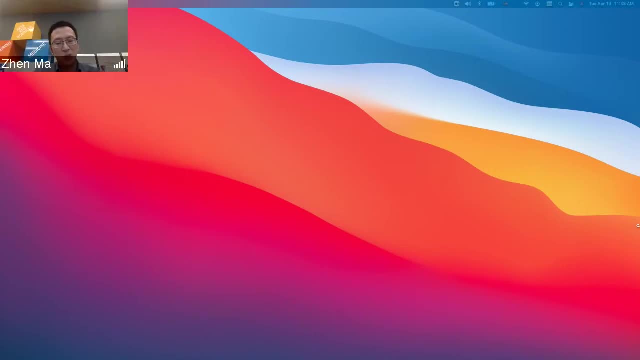 like some initial thought, why we have like stromal cell, like more on the bottom. So basically like our organoids is now cell floating in a matrix, right They are differentiated from micropattern in the colonies, which means the organoids basically get stuck. 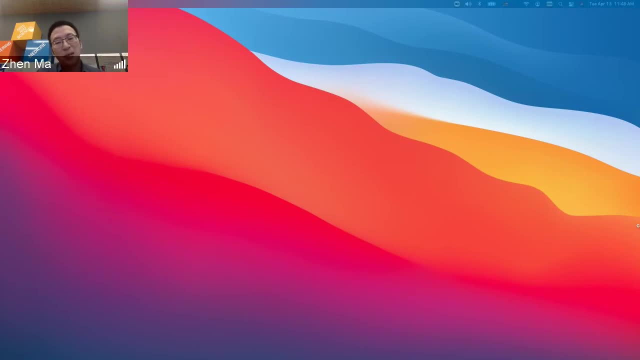 on the bottom of the substrate. So, and the substrate is very stiff, And then they need some cells that can holding up the entire tissue and stick to the bottom, And that was the stromal cells. So basically, the bottom layer is the stromal cells. 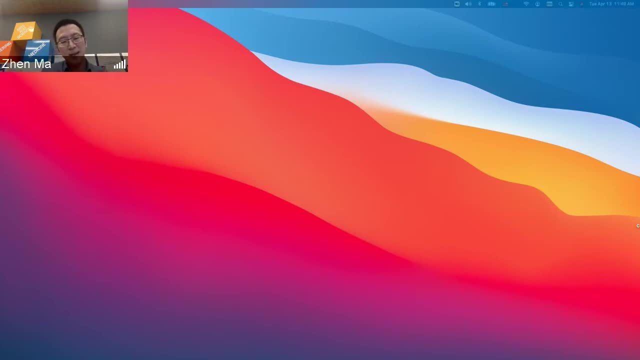 that can support the entire organoids And then on the top is much softer, the tissue much easier to contract, to move And that was best staff for the cardiomyocytes Because they need a contract. it's much easier to differentiate on the top of the organoids. 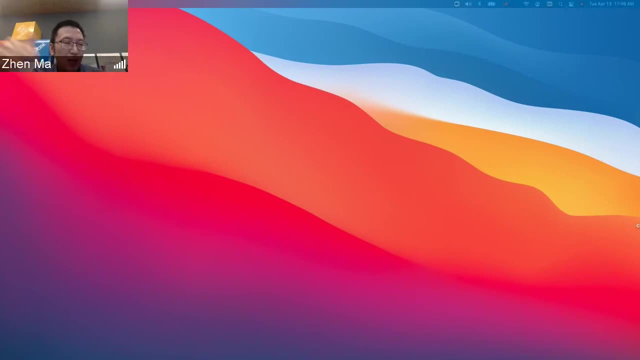 So, but of course I only take like more like a mechanical biology aspect of these spatial differentiations. There should be some signaling behind this spatial differentiations. But I can tell you, first thing is, when we do, we do some staining at the day four. 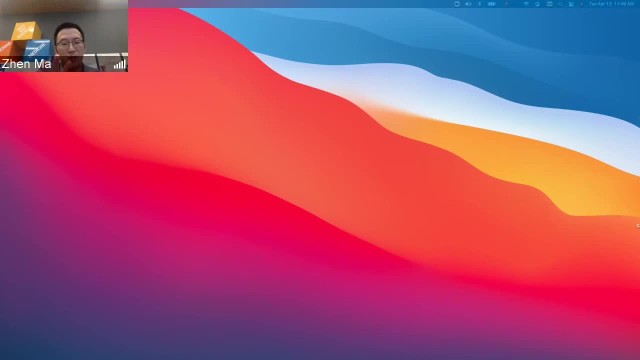 When the mesoderm and endoderm start to co-emerge on our organoids. Actually, the mesoderm cell and the endoderm cell, they are mixed together at day four, But when we do the staining at day 20,. 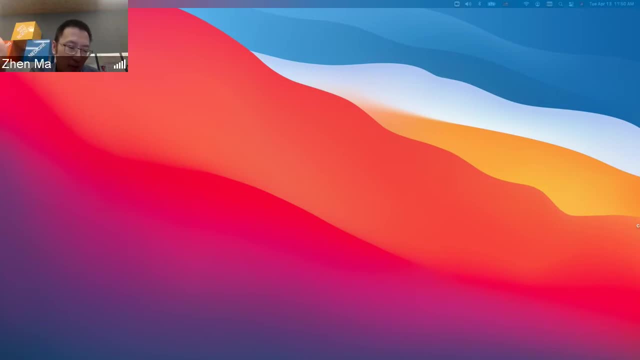 again using the cardiomyocytes plus as other, like endoderm markers for liver and some liver markers. So the spatial differentiation occur, showing up on the day 20.. So I don't know what's happening from day four to day 20.. 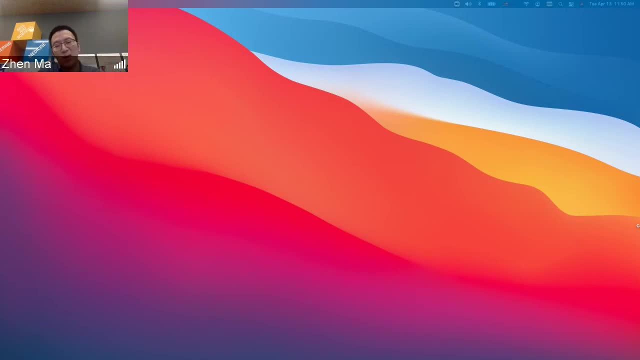 So at the beginning. so the endoderm and the mesoderm was mixture and they find a way to sort them out in that 16 days to the final product of the cardiac organoids. That's something that we are really interesting to looking at. 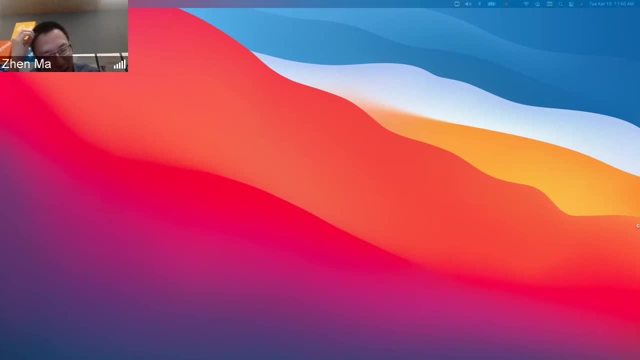 And we are currently, as I mentioned, at the endoderm. we're working with the endoderm and the mesoderm to really try to do the same thing. So, as I mentioned, I collaborate with a Costco lab and try to use some teleinformatics method. 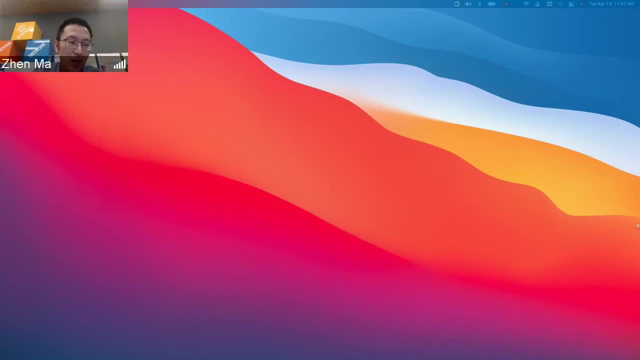 to try to see if there's a ligand receptor interactions between different cell types. That can probably can give us better ideas how this endoderm and mesoderm cross, talk each others, and to create that spatial differentiations. So here I posted the following question: 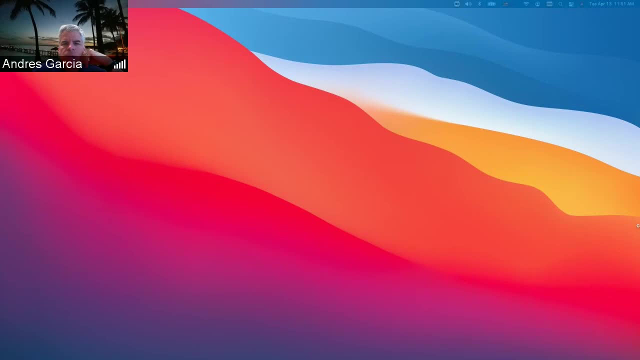 Beyond the cardiac formation and beating frequency, could you leverage your earlier data showing endodermal differentiation in some organoid sizes to study drug effects on this development or how it interplays with cardiac development? So that's really a great question. It's something what we really want to do. 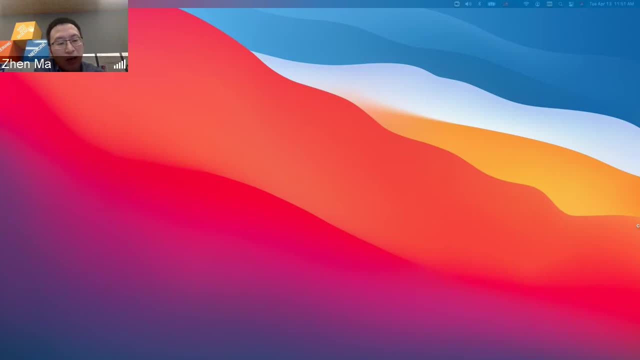 In development right heart and liver. they are co-development. Heart is slightly early than liver, but basically, like a liver, like heart, send a lot of signaling- BMP signaling to the liver and the liver like pay back a lot of FGF signaling to the heart. 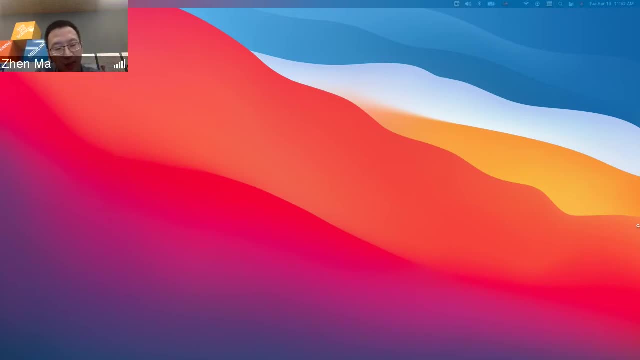 So there's a lot of cross-talk between the heart and livers during the development. There's something we really want to do and looking at. So one thing I like to highlight is also from our data- I didn't show here there are some population of the cells in the endoderms. 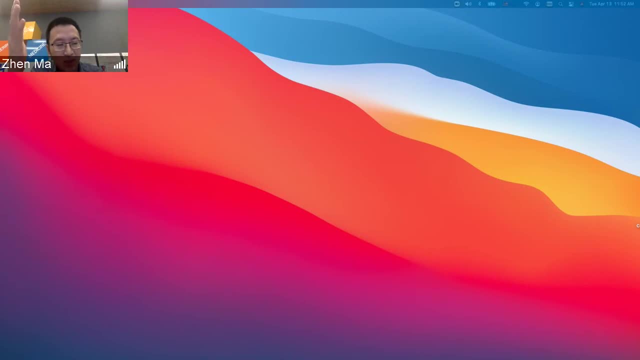 They're actually expressing some genes is inhibits the cardiac differentiations. So I think, like in our this, like Organized, they have to find sort of a balance between the mesoderm and the endoderm so they promote each other at the same time they also inhibit each other. 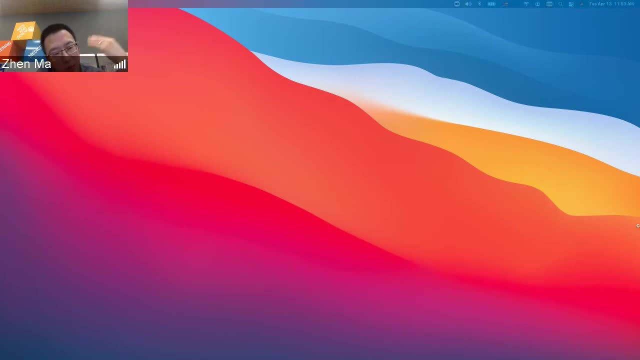 I cannot say each other, because our protocol is primarily drive to the cardiac differentiations. So maybe the immersion of the liver, the immersion of the endoderm cells will play a role. try to slow down or reduce the protocol. So maybe the immersion of the liver, the immersion of the endoderm cells will play a role. try to slow down or reduce the protocol. 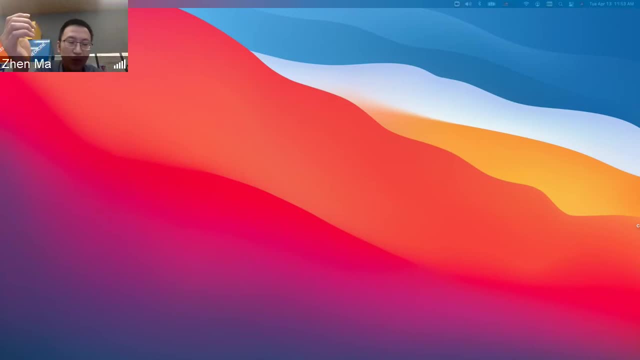 So maybe the immersion of the liver, the immersion of the endoderm cells will play a role, try to slow down or reduce the protocol. So the cell- I think it'solie gene感じment has betteroris, regardless of organ États, is something that can be treated. 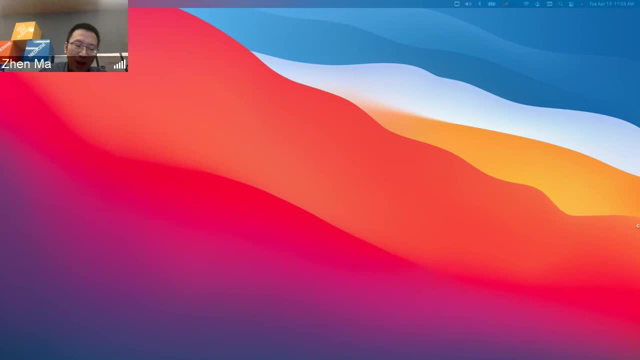 If I can use in some magic way that can totally remove the endoderm like cell differentiations. So if I can use in some magic way that can totally remove the endoderm like cell differentiations, maybe I have an even better cardiac Ziggo functions for our organoids as well. 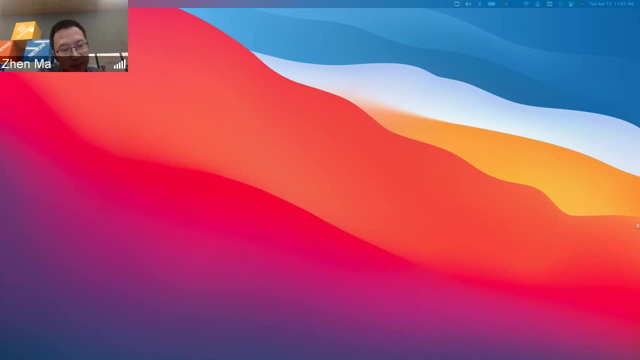 Maybe I have a even better. cardiac Ziggo functions for our organoids as well. Okay, So another question: The cardiac organoid 3D model is different from with valvular descent or expansion, and gas transfer. the cardiac organoid 3D model is different from with valvular descent and gas transfer. 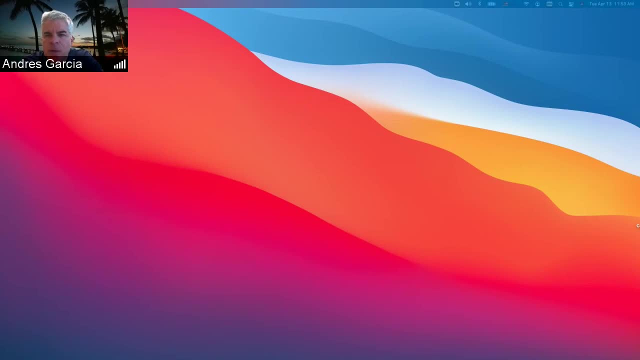 Okay is very useful for drug screening. We are developing drugs targeting tropomyosin isoforms, such as TMP3.1, which regulate the functions of specific populations of acting filaments. Since TMP3.1 is not a muscular isoform, do you think your model can be used to test? 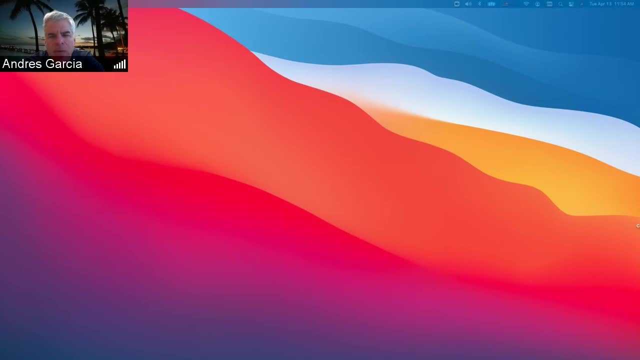 these anti-TMP3.1 drugs to validate that they have no impact on cardiac functions. I'm sorry, I think I lost a little bit. I didn't quite get the half part of your. So they have drugs that target tropomyosin isoforms, such as TMP3.1.. I don't know how. 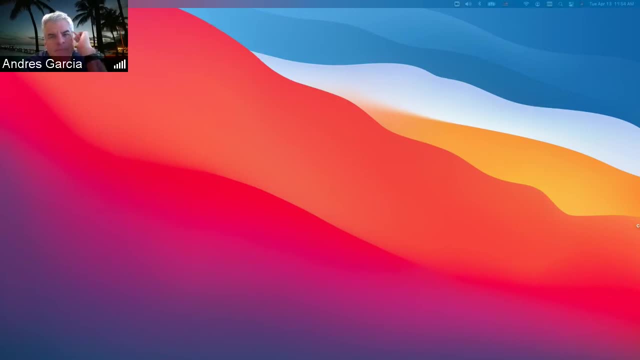 to pronounce that, But that tropomyosin is not a muscular isoform. So do you think you can use your model, your cardiac 3D model, to test the drugs to validate that they have no impact on cardiac function? I think yes. There has been many different models that can be used for testing drugs. 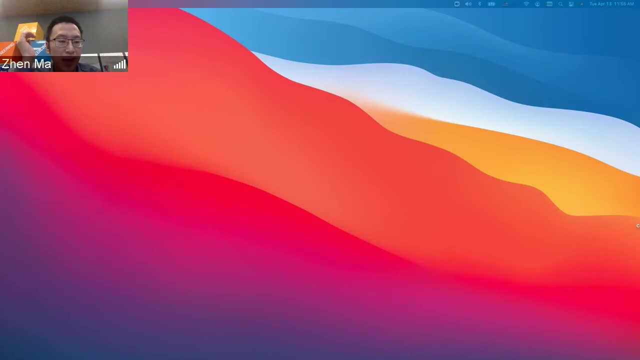 or the disease modeling. I think that's a very interesting aspect. So at the very beginning of the talk I do show we have another model- we call it micro tissue models- which try to recreate the cardiac muscle that's more similar to the heart, which is highly elongated, and the uniaxial contractions. 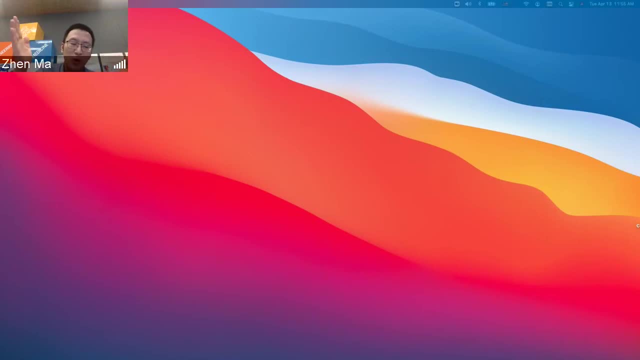 And on that platform we can measure the force as well. So for the organism we can now measure the force. So I think for a lot of cardiac responsive drugs normally we go to that model instead of ordinary models. But I'm happy to let the conversation roll in to using our other models to 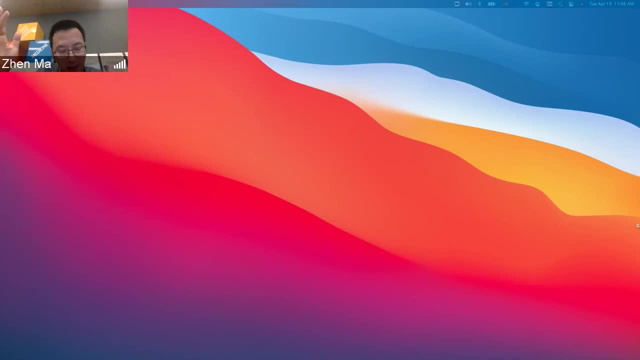 give a test on the drugs, how the drugs will modulate the contractile functions over the cardiac microtissues. Okay, The next question is from Professor Eric Driden. Regarding translation of your teratogenicity assay, I'm curious what future studies will be required from confirmation Human trials. but that 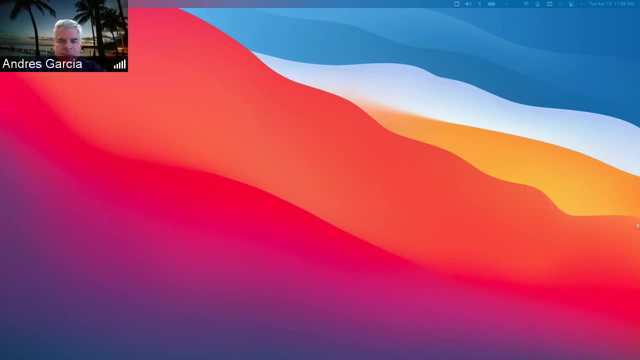 probably would be a difficult sell. So you mean for the neuro toxicity- Yeah, I think it's for the, yeah for your assay of teratogenicity. So so currently, like, this is my like R1 grant. So basically my R1 grant is just: 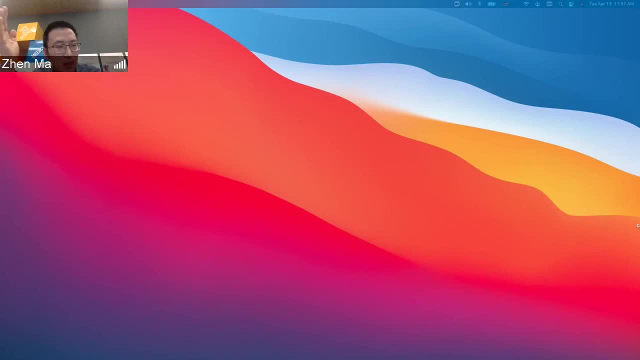 trying to use this model to establish like a biostatistic model. So basically, if you have a new drug, we can feed in the model mirror the data using our cardio-organized and feeding in that static model, and then the model can tell you what's the risk level of embryo toxicity. 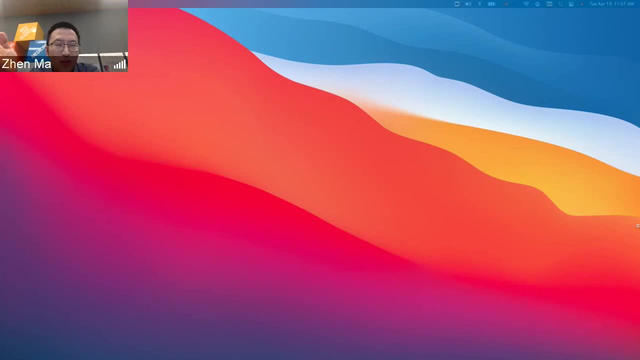 So, and this is how pharmaceutical companies using their mouse model in their research. So it's, I think, like in terms of this: how's the progress? right, I think people should be taking like one step forward, but now, like directly, go to the endpoint, like to humans, to compare. 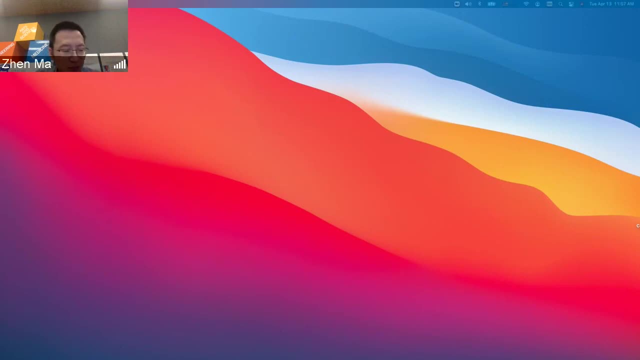 So I think, like for a near future, what I really want to do is just compare so many different models for embryo toxicity, not just the physical model and also the computational models, with, like the risk classification systems to determine which one has a better predictive activities. 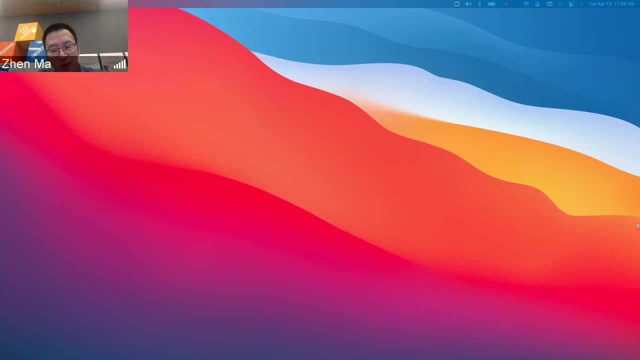 right Which have more precisions on the embryo toxicity screening. So I just don't think eventually like this is the way people can do a lot of human trials with the pregnant women's right. So, for like for vaccinations, pregnant women should be excluded. So 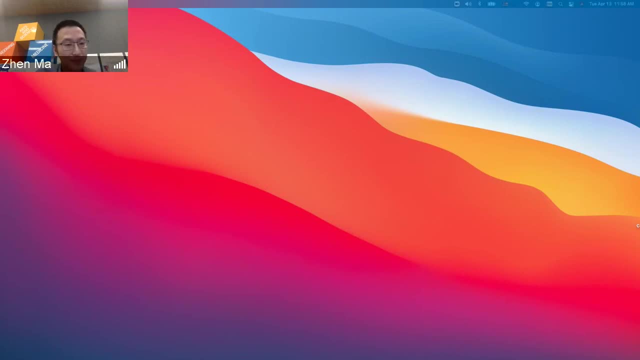 just not a way to do it. Okay, And we'll take the last question is from David Wolfson: Do you think it would be possible to leverage your single-cell RNA-seq data and DERP screening platform to find differences in cardiac chamber or phenotype specific responses? 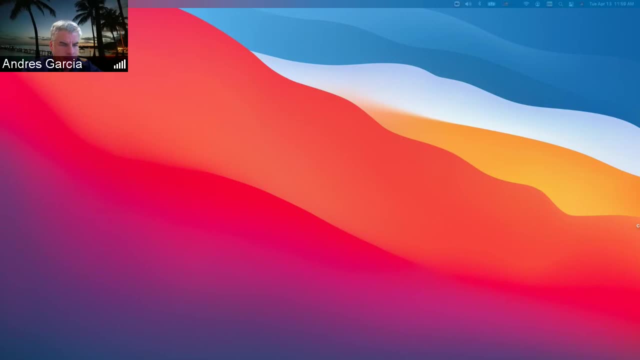 Yeah, so in our research the single-cell RNA-seq is very, very expensive. We are going to do a lot of screening and we're going to do a lot of analysis to experiment with single-cell RNA-seq to see if there's a difference between the two. So I think like the single-cell RNA-seq. 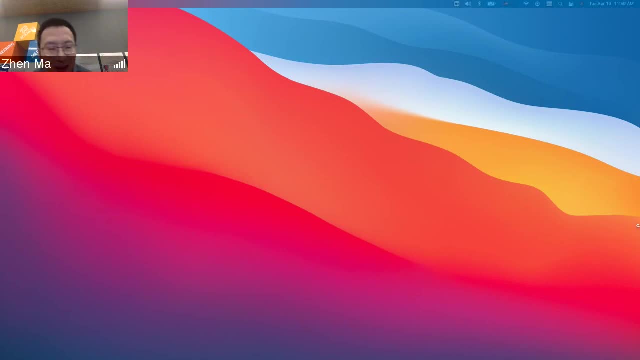 open up a lot of possibility for us. So by the other side. so this experiment is very expensive. We are now planning to do all the screening, or transcriminal analysis, using single-cell RNA-seq. Okay, We're currently actually doing a lot of bulk IRN-seq as well for drug screening applications.